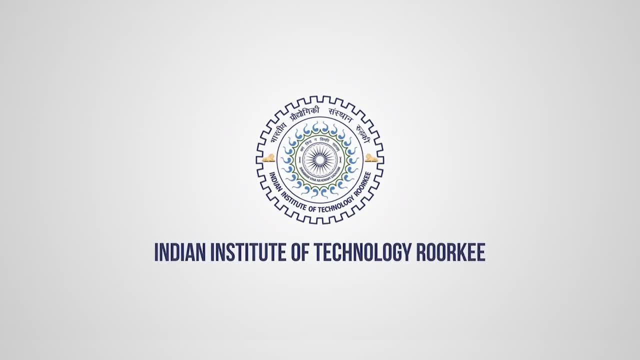 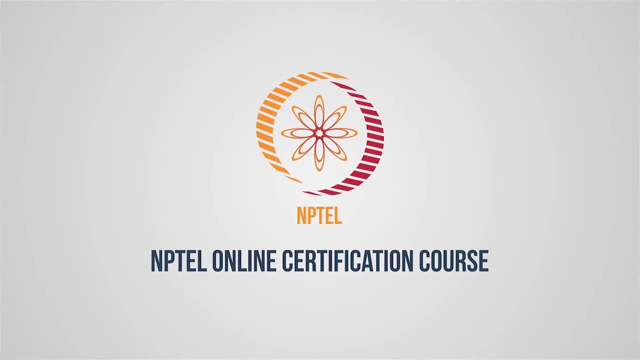 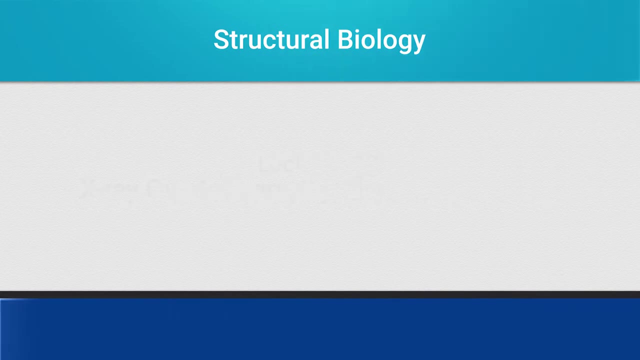 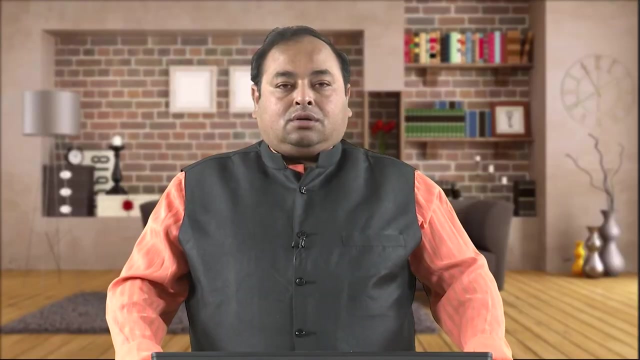 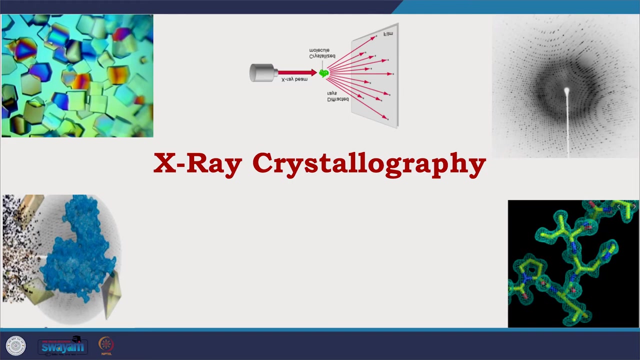 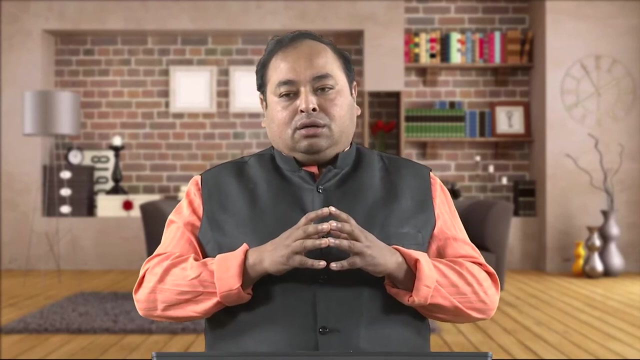 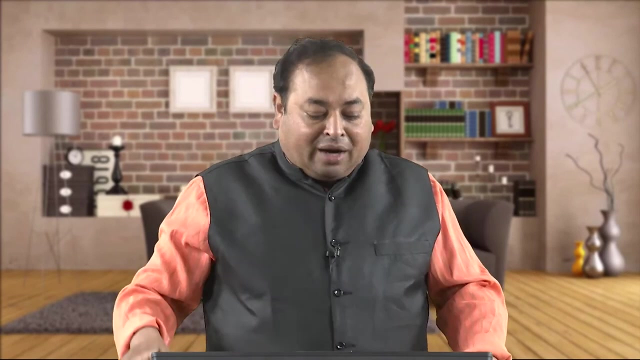 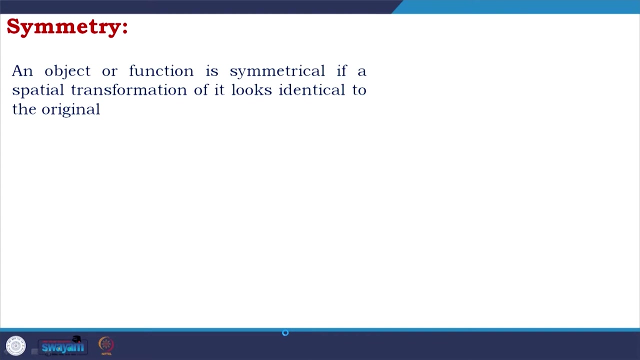 Hi everyone, Welcome to the course of Structural Biology Today. this is an course on the continuation, where we will discuss about symmetry as in a overall concept and symmetry in crystallography. So what is symmetry? Symmetry is called if an object or function 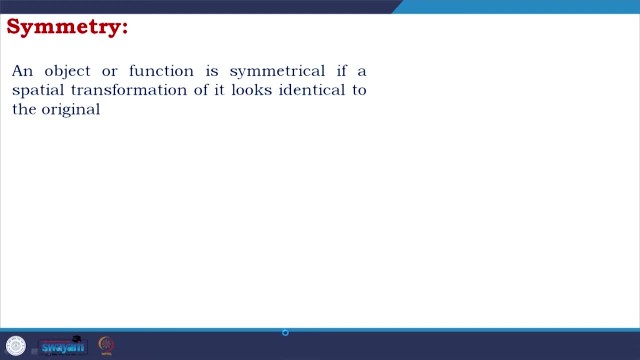 is symmetrical if a special transformation of it looks identical to the other. Symmetry is called if an object or function is symmetrical if a special transformation of it looks identical to the other. Let us say this: x is original. Now, if I make a 180 degree rotation and come to this, then 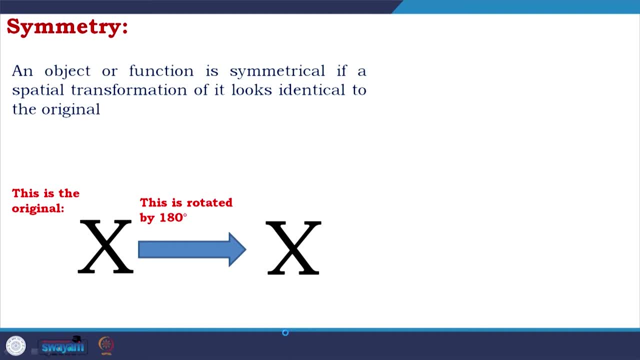 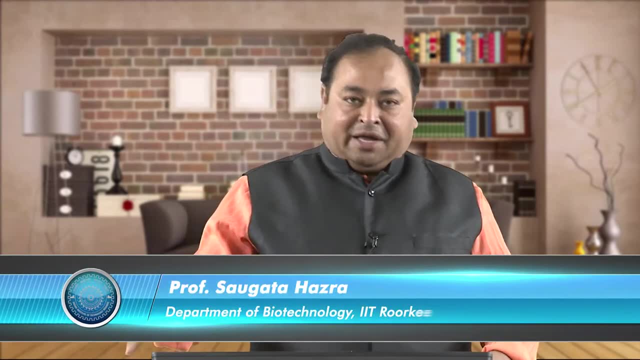 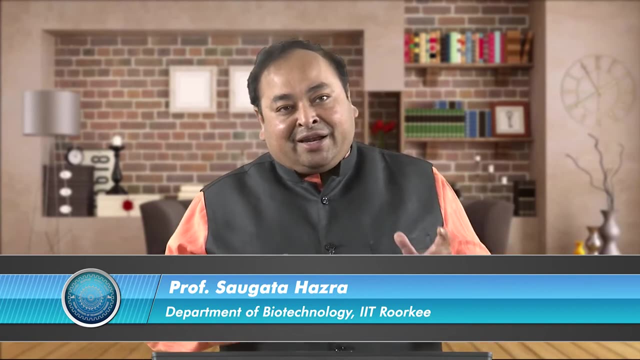 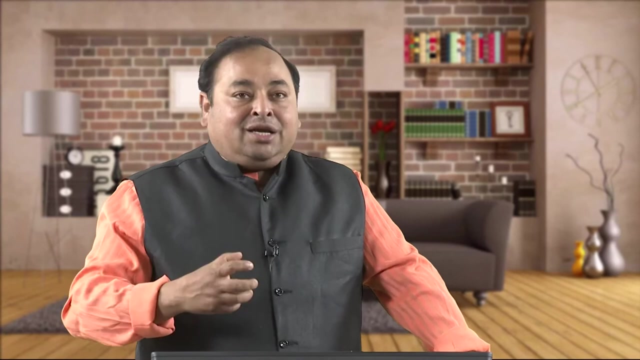 I would say it is symmetry. But the interesting case is, if you see, you know that there is a 180 degree operation made, but because of the symmetrical nature of the structure you do not understand it is a 180. So what we need to see symmetry, we need a standard with respect to the standard, your. 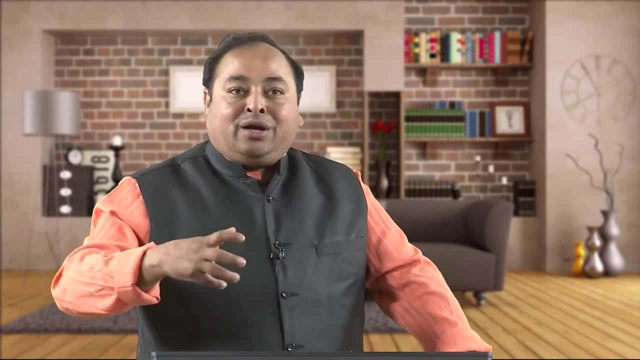 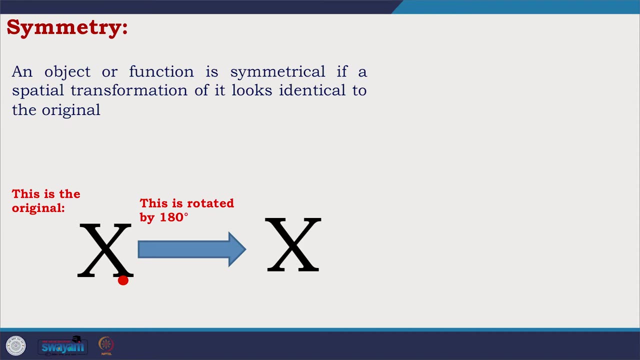 symmetry would be more pronunciably, more clearly understood. Let us say, I put a red dot here, and now, when I perform 180 degree, you see that the rotation happened. and now this comes here. The red dot is not part of the system, not part of the symmetry, but 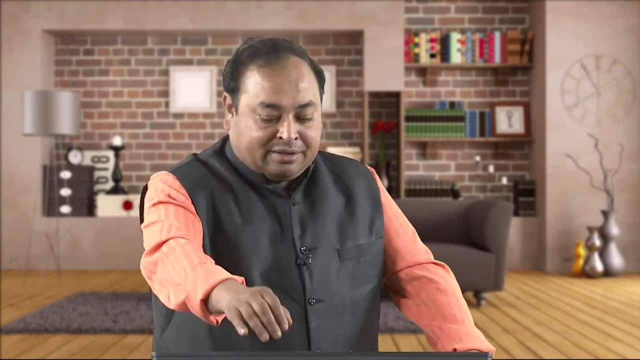 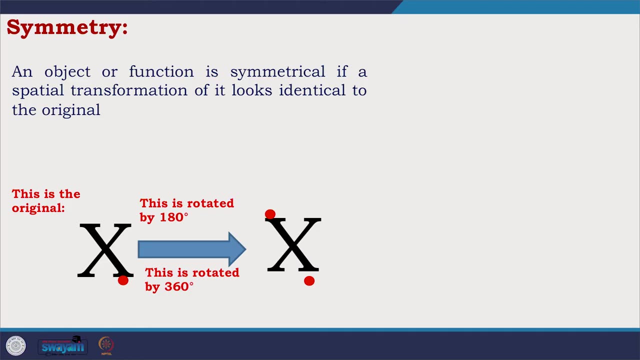 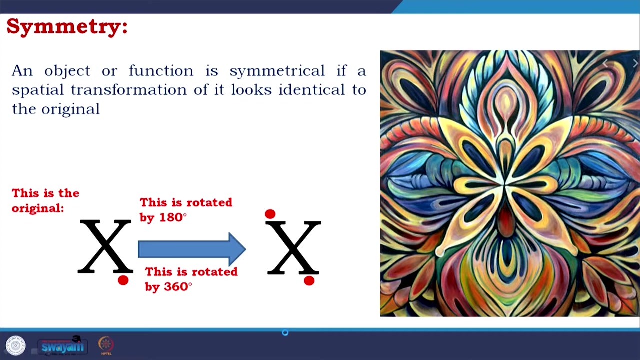 the presence of it makes yourself clear. Similarly, a 360 degree rotation now would bring it here. This is a complex symmetrical representation where there are symmetries in some portion. some are not symmetrical. So I have tried to put you know, dotted white line, if you see. 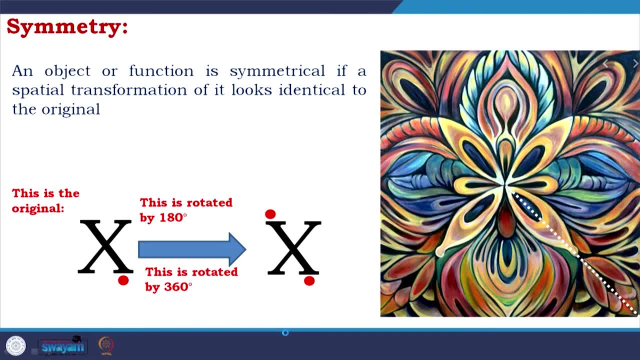 on the screen, you will see that this part and this part are symmetrical. So you see symmetry here. you see symmetry here. you see symmetry here in that way. Similarly, you get symmetry here because it is a hand drawing. So the symmetries are. 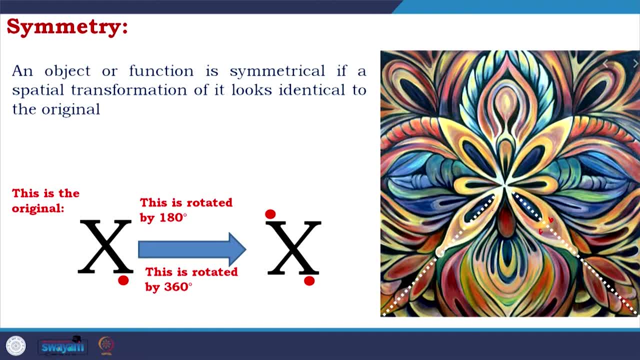 not as perfect as we get here, But you clearly realize the symmetry. Similarly, here there is a symmetry, here there is a symmetry. but if I compare between these and these, they have a similar pattern but they are not similar. they are very different. There is symmetry. this side there is symmetry. 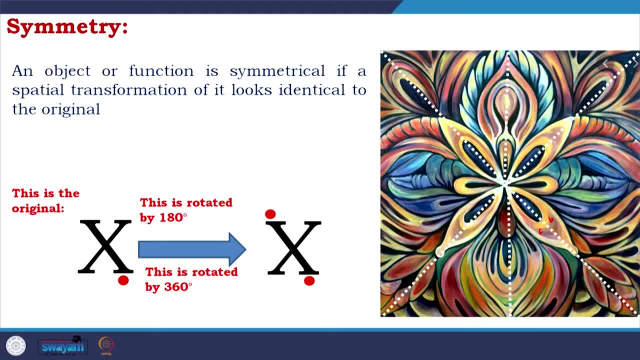 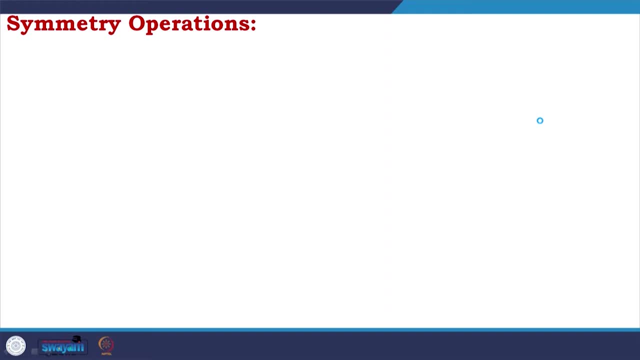 between. Again, if you see, the symmetry is here, the symmetry is there, But there is symmetry here, but between this part and this part you do not get the symmetry. So this is kind of a presentation where you know, we get complex drawings and all. 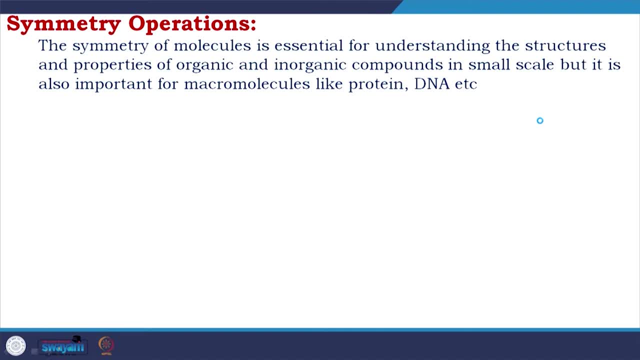 What is symmetry operation? The symmetry of a molecules is essential for understanding the structures and properties of organic inorganic compounds. where we are talking about small molecules important for macromolecules like protein DNA specially, we are studying X-ray crystallography. 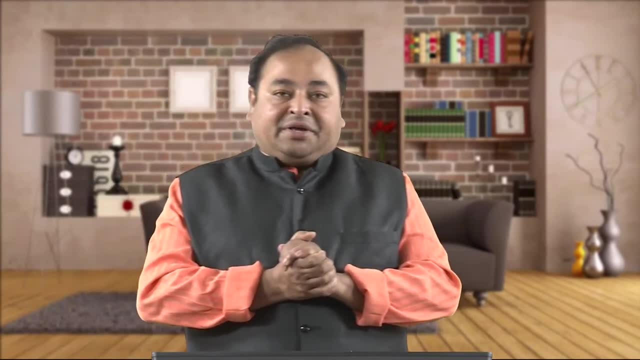 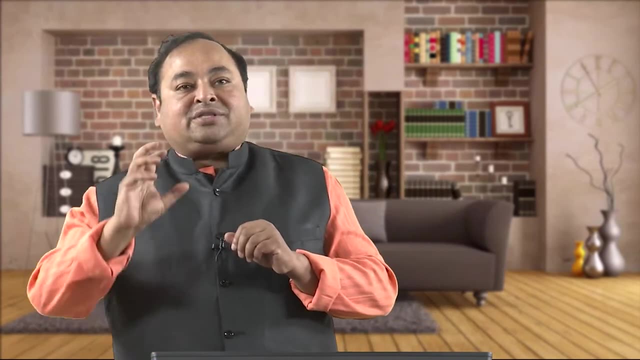 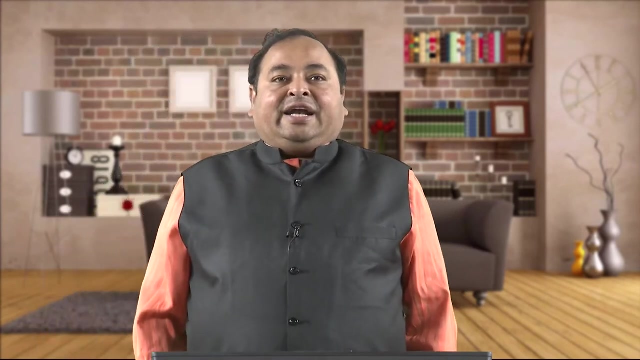 you will see that, the presence of symmetry. so I will tell you: there are two type of symmetries: one is crystallographic symmetry and other is non-crystallographic symmetry. What is non-crystallographic symmetry? Let us understand first. if I am standing here, a line could be drawn here, so there is clearly. 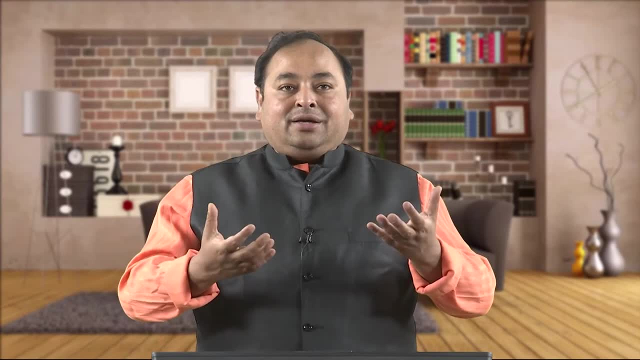 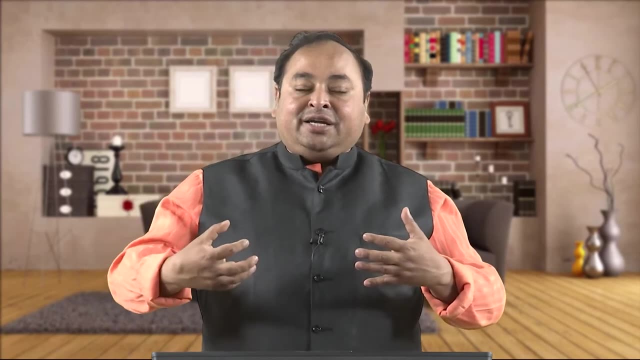 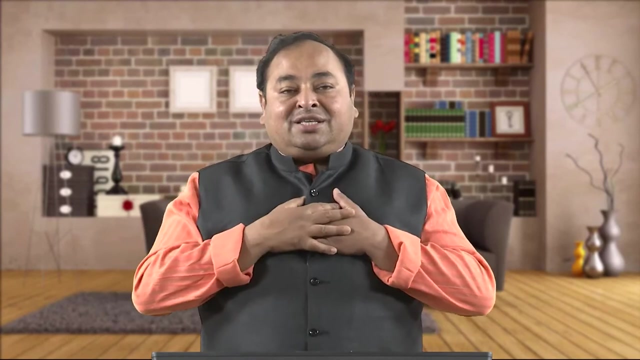 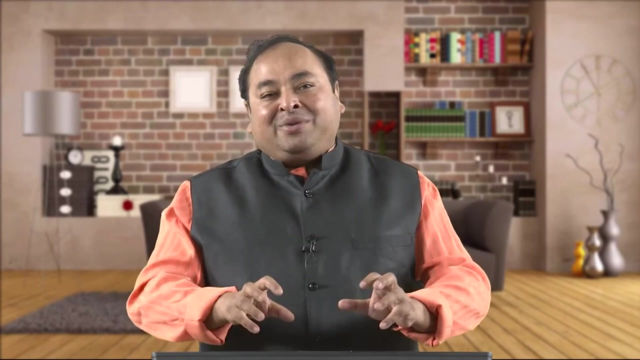 two homogeneous, or you say symmetrical part which form my body. that is what nature did. it did not come through the technique of crystallography or the technique of other symmetry operation. so this is natural symmetry, non-crystallographic symmetry, Something which comes when the atom is arranged in the crystal lattice. that is crystallographic. 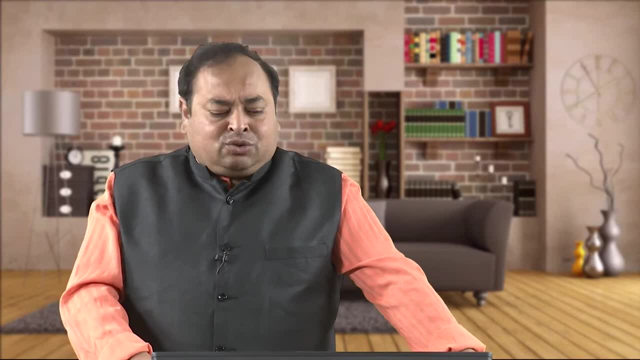 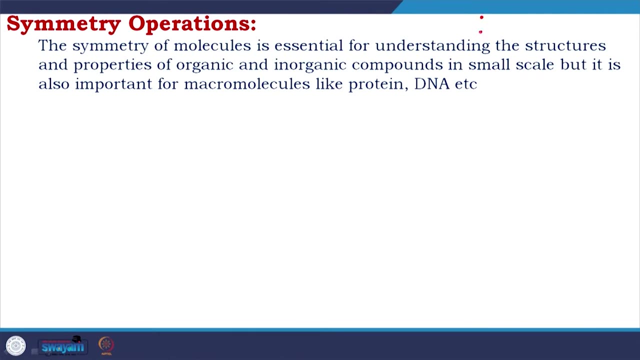 symmetry. Why? it is very important to understand. just see this: you have a crystal where these dots are in identical positions. So what you could do: You could take one of these dots, You could take one, but by solving the structure of the motif 1, you could apply symmetry operation. 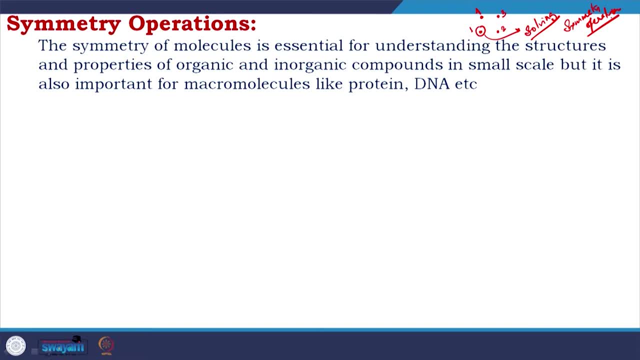 then you do not have to solve 2,, 3 and 4 individually, So your work is symmetrical. So what is non-crystallographic symmetry? That is the beauty of symmetry and its role in crystallography. 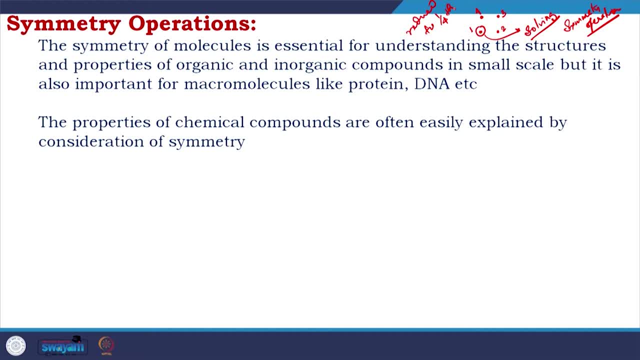 The properties of chemical compounds are often easily explained by the consideration of symmetry. Let us take an example. the symmetry of a molecule determines whether the molecule has a permanent dipole moment or not. sometime we see molecules right, like a water molecule, like a carbon molecule. 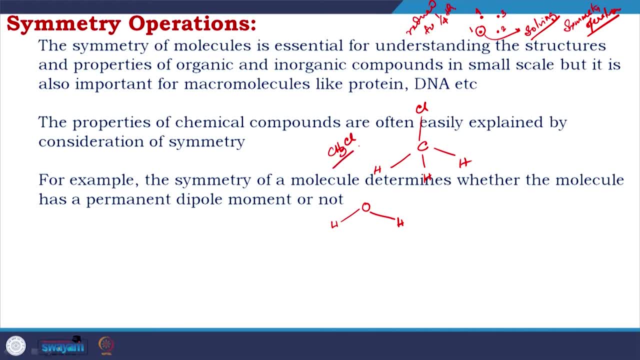 being CH3Cl and a carbon molecule being CCl4 or a carbon molecule being CH3Cl. So in this way, the set of carbon molecules would have different dipoles based on their symmetry and positions. The theories that describe optical activity- infrared and ultraviolet spectroscopy- and 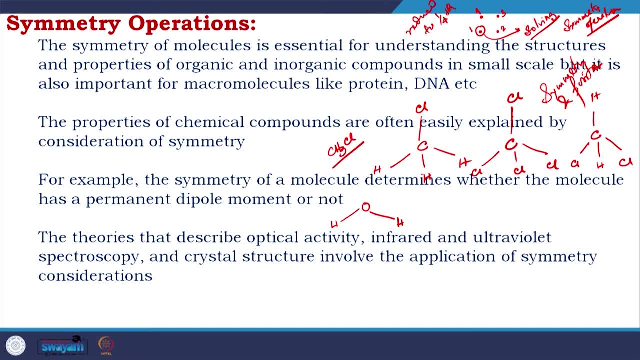 crystal structure involve the application of symmetry considerations. the stretching, If you see, in carbon dioxide in normal condition, but because the directions. but if the directions are, If it is stretched, Then. So this is the generation of dipole Matrix. algebra is the most important mathematical tool in the description of symmetry and we 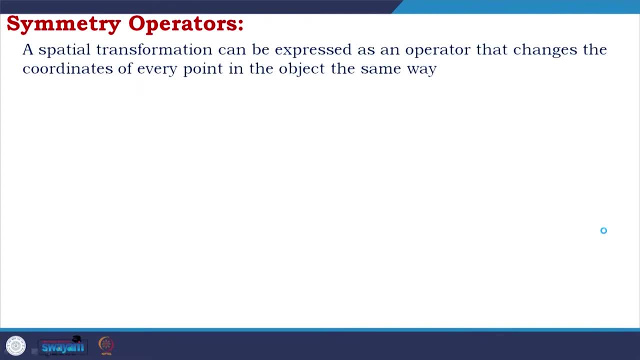 will see some of the operations. So, coming to the symmetry operators, a spatial transformation can be expressed as an operator that changes the coordinates of every point in the object. the same way, Symmetry operators, Symmetry operators, Symmetry operators And distort the object. 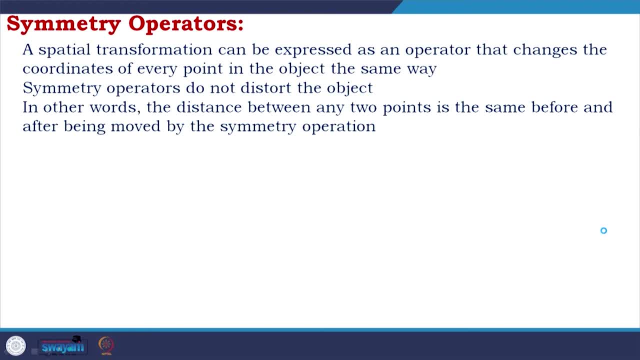 In other word, the distance between any two point in the same before and after being move by the symmetry optimization would be identical. Here is the operator for a 180 degree rotation around the z-axis. So you see the around the jade axis. it is the operation happened. 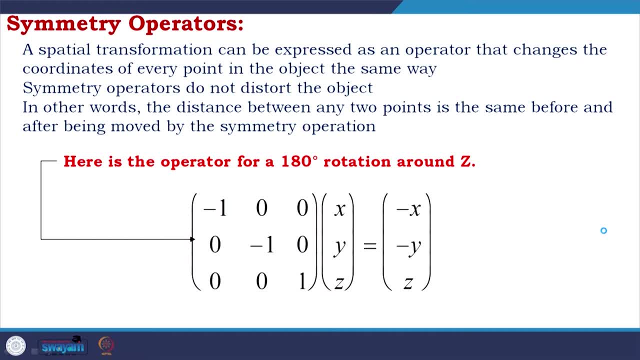 So x and y, There are changes And also due to all that change with the force changes x, y z minus x minus y z. So these two are equivalent positions and the concept come from 3 into 3 matrix multiplication which have a matrix form like this: 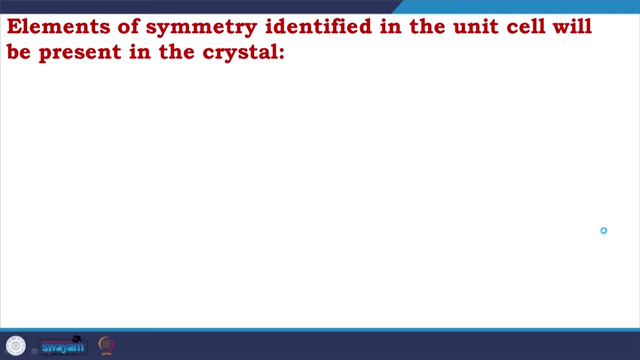 The elements of symmetry identified in the unit cell will be present in the crystal. so which would be the symmetry one, the centre of symmetry, which we call inversion, Rotation mirror, which is reflection. we will talk about them. Translation- translation is movement and glide, which is a combination of reflection as well as translation. So they are all referred. 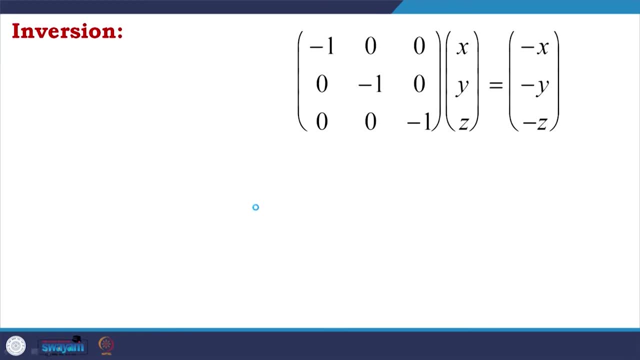 to as symmetry. Now let us see the symmetry inversion where, if you see, all the coordinates are change, x, y, z converted to minus x, minus y minus z. So there would be a point and if you measure, every position would be equidistance from that. So if this distance is this, this distance, 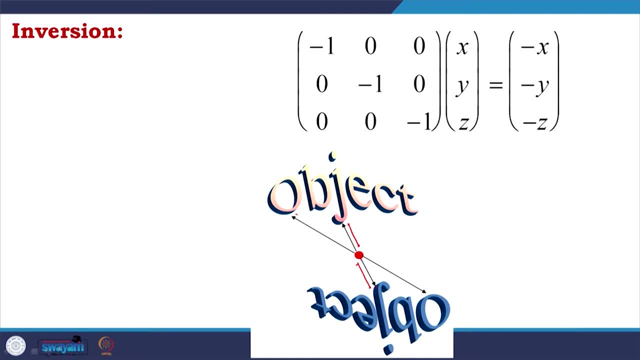 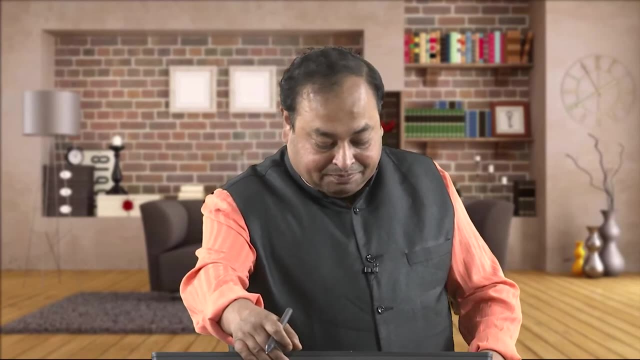 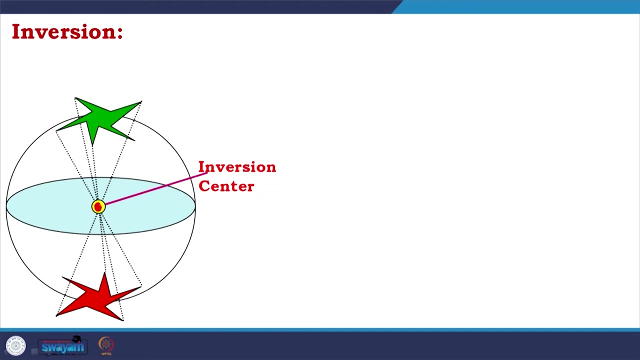 distance would be same. similarly, this distance and this distance would be same. So inversion provide a point from where everything inversed. Here also, this is talking about the same thing. we have a point here and from that point is acting as a inversion center. all the distances are identical. 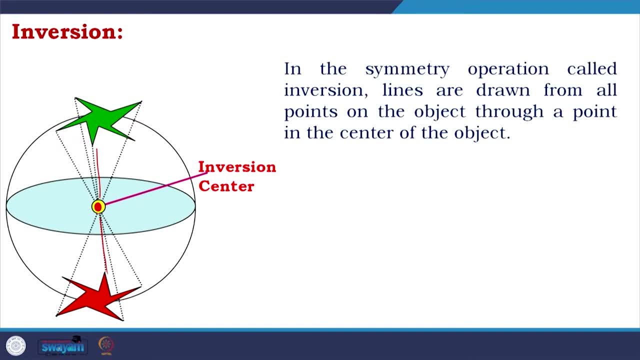 So in the symmetry operation called inversion, lines are drawn from all point on the object through a point in the center of the object, which called inversion center. This is called a symmetry center and it could be symbolized. It is also called inversion center, as I told. 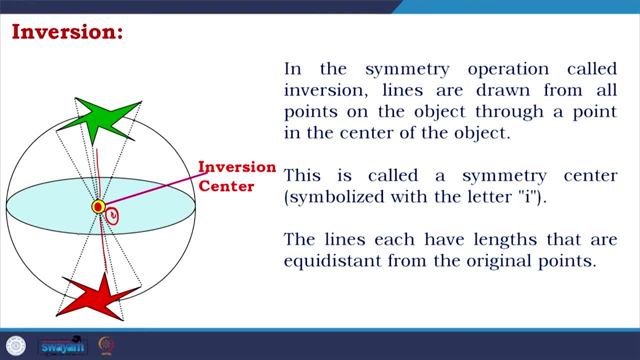 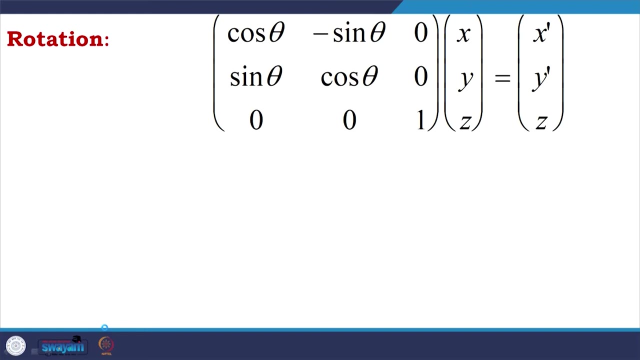 The lines each have lengths that are equidistant from the original point. So each of the points here from this point would be equidistant from the 2 objects which we get from inversion operation. Coming to rotation, here, In rotation We definitely have angles. 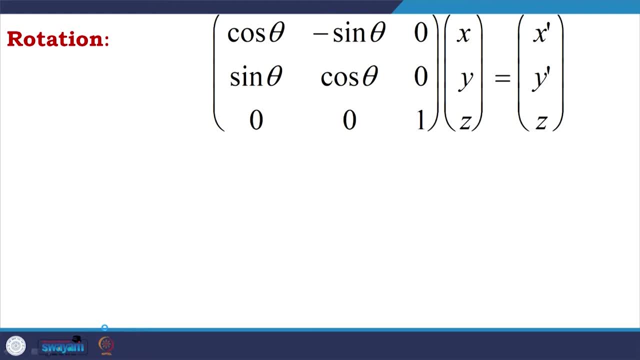 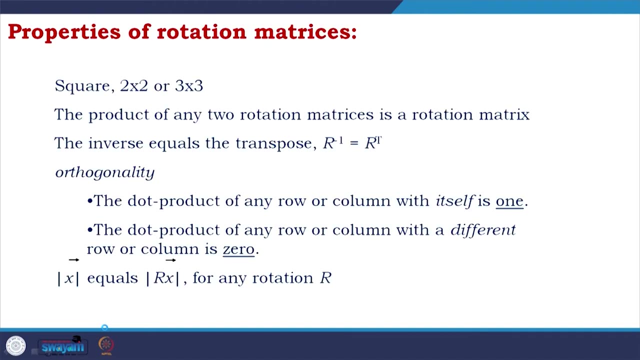 So X, Y, Z, that is, change in according to the X and Y axis. So this is a representation of rotation. in the rotation matrix it could be 2 in to 2. for 2D it could be 3 in to 3, because in case of rotation, as we have seen here, 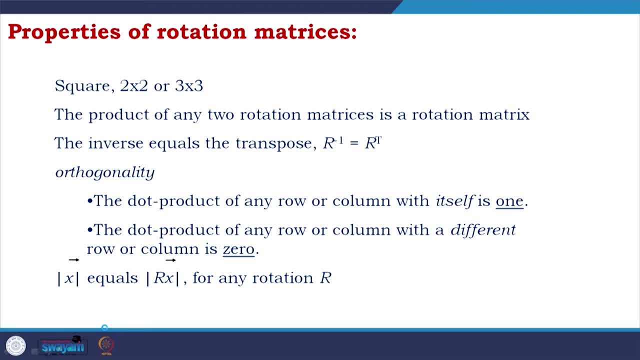 This is 2D be 3D also, which we will see. the product of any two rotation matrices is an another rotation matrix: the inverse equal, the transpose. So R inverse equal to R transpose. it maintains orthogonality. the dot product of any row or column in the matrix with itself is one, the. 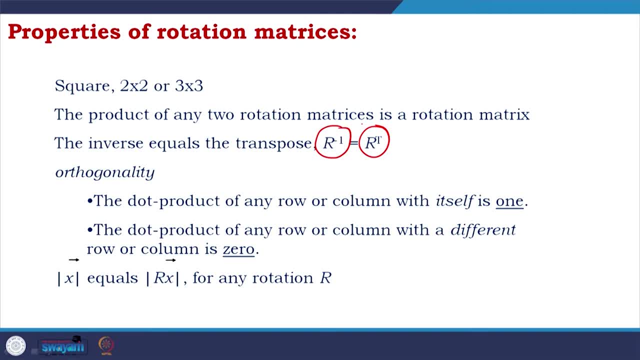 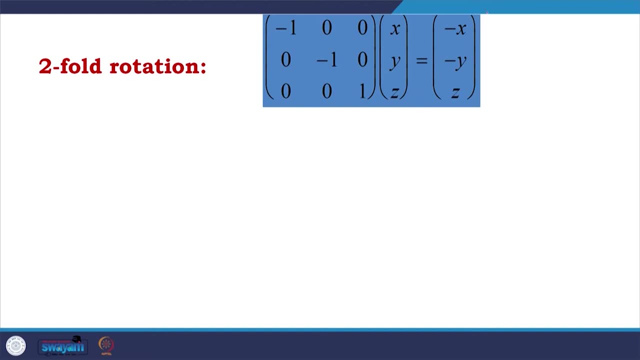 dot product of any row or column with a different row or column is 0.. The vector x: its absolute value equals to R x for any rotation, R, Two fold rotation. here you see change in the two axis. So this is a representation of two fold rotation which maintains phi 2 symmetry. 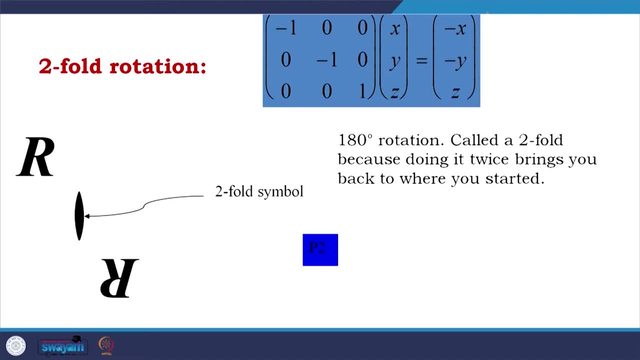 It is a 180 degree rotation. It called a two fold because doing it twice brings you back to the original where you have started. So two fold axis here to here. the difference when you see rotation with reflection is the change. So it would be. 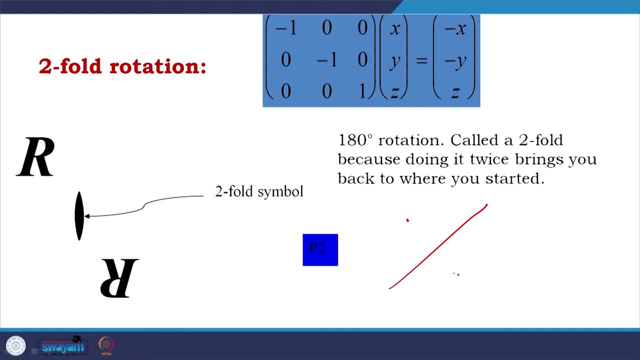 see the point from where the performance of rotation have operated equivalent position in fractional coordinates. I will explain what is fractional coordinate. is x, y, z minus x minus y, z would not be there, So z would be z, other two would be change threefold rotation. 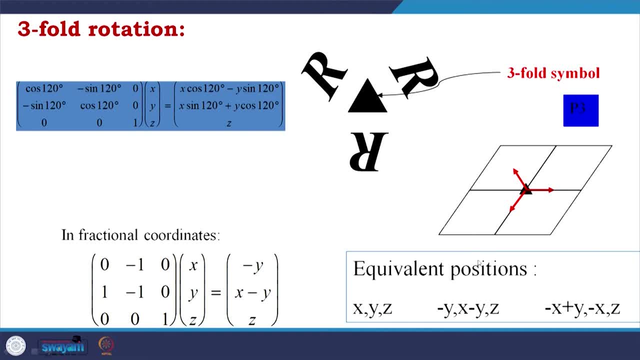 as you see in the matrix. here you will see the changes and in the fractional coordinate you will see from x it is converted to minus y y to x minus y z is not changed. It represent P 3 symmetry. the equivalence positions are x y z minus y z minus y z. 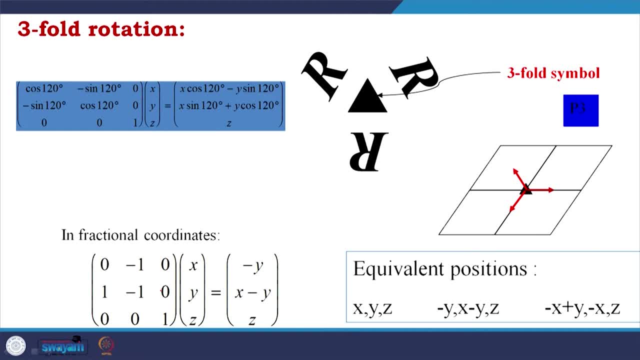 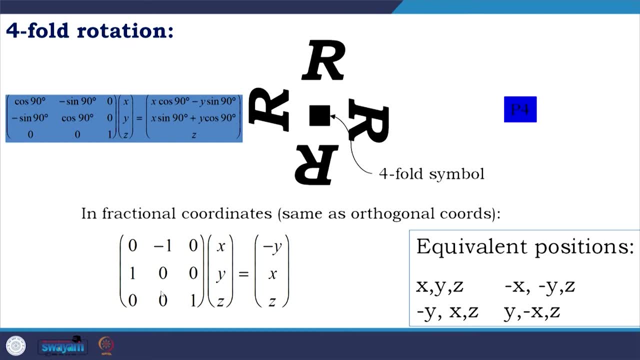 Minus y, x, minus y z, minus x, plus y, minus x, z. fourfold rotation: again it is a P 4 symmetry. So if you see x y z, it is changed to x, changed to minus y. So the position change, y change. 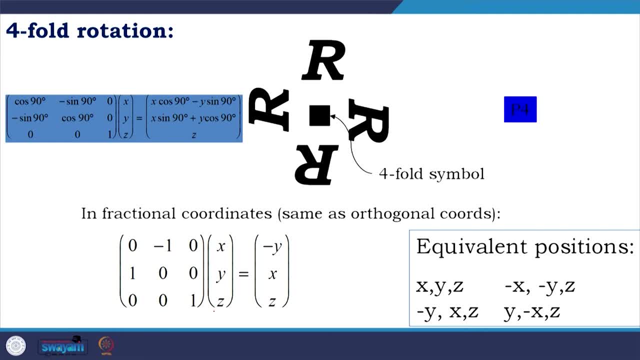 to x and z would be taking as z. So it is fourfold means it is 90 degree, So it is 90 degree. when it was 3 fold it was 120 degree I will talk about. but if it is 6 fold then it is. 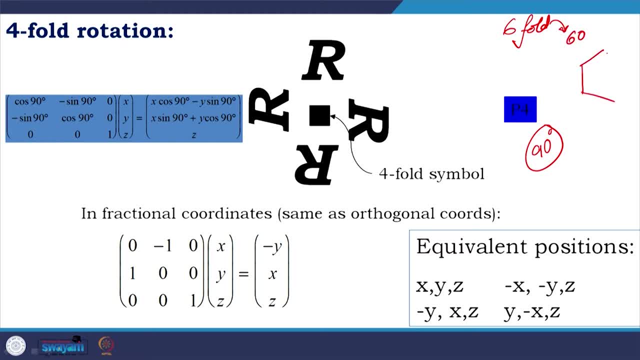 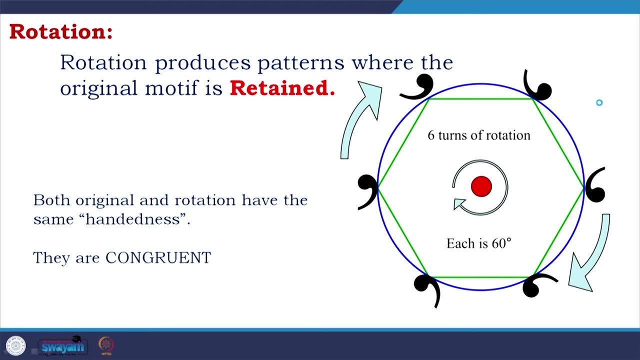 60 degree like a hexagonal or a benzene ring Rotation produces patterns where the original motif is retained. If you see the original motif, as I was talking about the hexagon here, in each case it is a 6 fold. So 60 degree rotation and both original and rotation have the same handedness and they 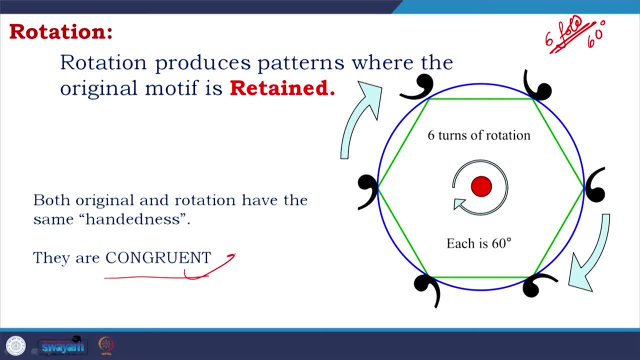 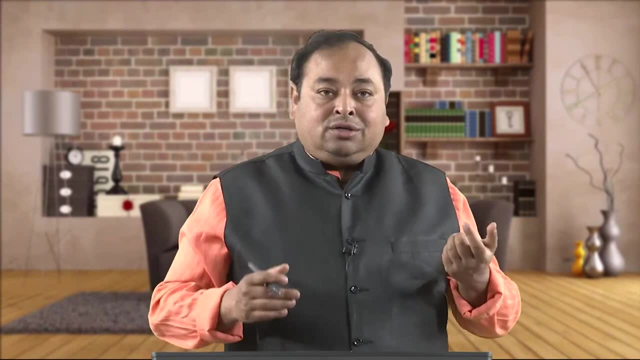 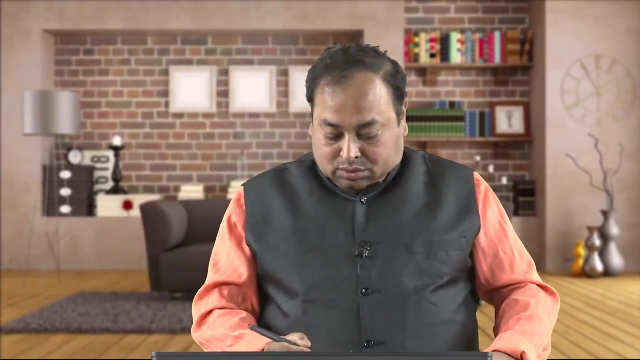 are congruent. What is congruent? I am going to explain it later, when the perspective will come, you will understand it even better. So we have two types of rotation. Two fold- we obviously have one fold, the same thing, two fold, three fold, So 1,, 2,, 3,, 4,. 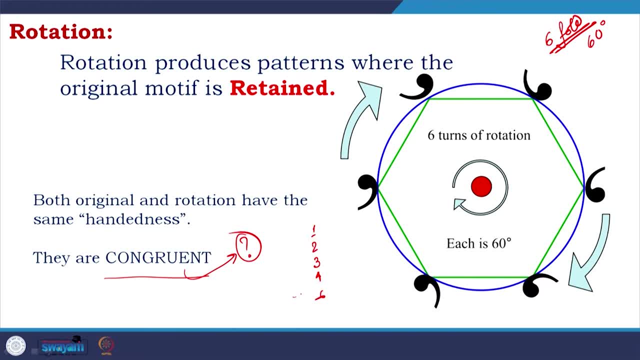 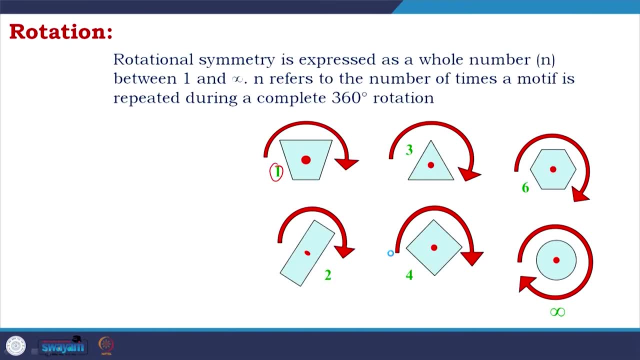 6, 5,? what happen to 5?? Again, we will see that Rotational symmetry is expressed as a whole number n between 1 and infinity. N refers to the number of times a motif is repeated during a complete 360 degree rotation. 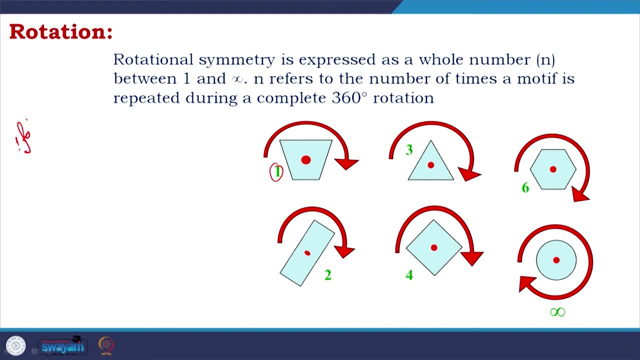 which means, if it is 1 fold, it is 360 degree. divided by 1, the rotation 2 fold the rotation is 360 degree. divided by 2 is 180 degree. 3 fold 360 degree divided by 3, which is 120. 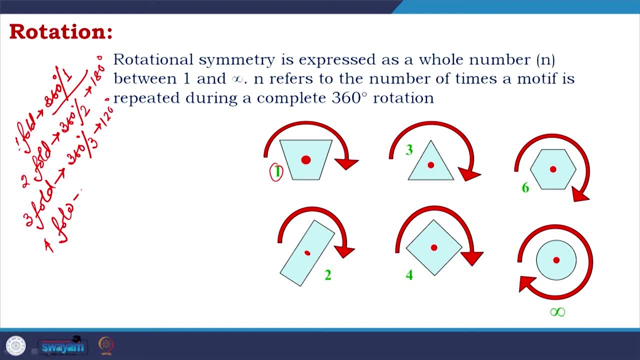 degree 4 fold 360 degree divided by 4 is 90 degree. 5 fold 4 fold 4 fold is 90 degree. If you have an idea is 72, 6 fold 360 degree by 6, 60 degrees. in that way you will get: 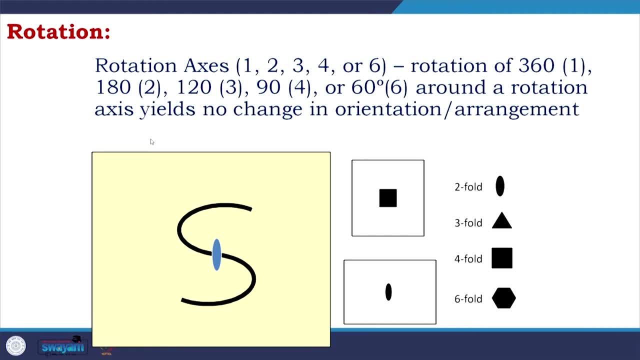 Rotation axis is 1, 2, 3, 4 or 6. rotation of 360 degree, 180 degree, 120 degree, 90 degree rotation axis yields no change in orientation or arrangement, As I talked about. if you see, here you are rotating, you are further rotating, you are. 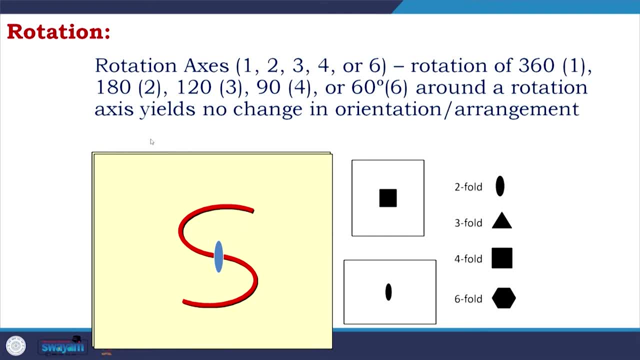 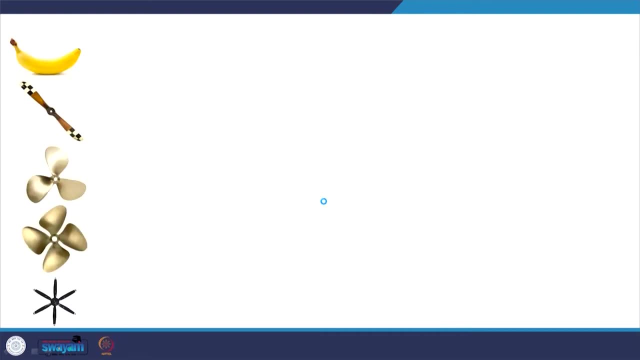 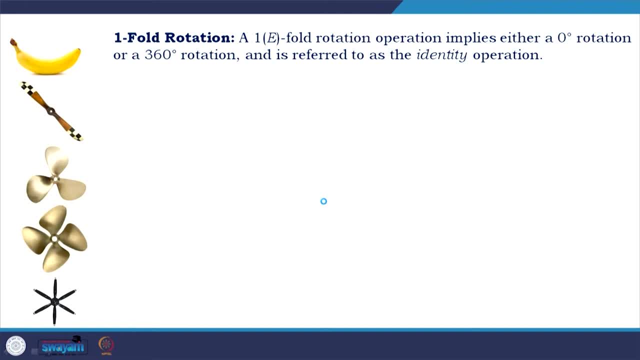 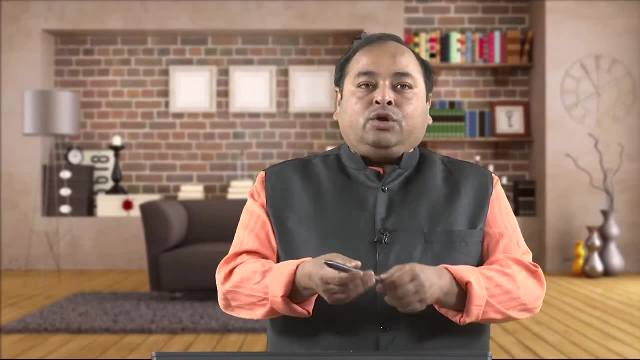 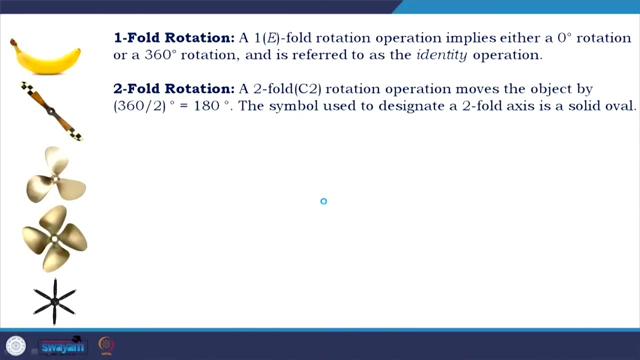 and is referred to as identity operation. so you have no symmetry. but if you take or you did not change, definitely get the same. you make a 360 degree change, you definitely get the same for anything. So this is one fold, Two fold rotation. a two fold is C2 rotation operation moves the object. 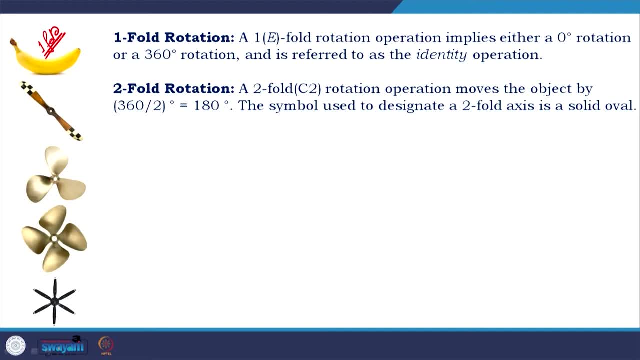 by 360 by 2180. the symbol used to designate a two fold axis is a solid oval. If you see, this is two fold, Three fold rotation. a three fold or C3 rotation operation moves the object by 360 degree, by 3120 degree. the symbol used to designate a three fold is a solid equilateral. 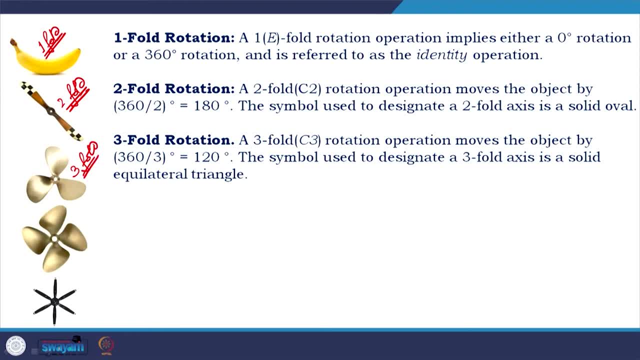 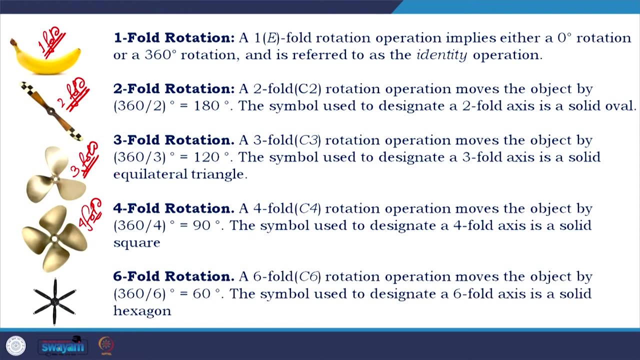 So here three fold. Four fold is C4 rotation operation moves the object by 1980. the symbol is a solid square. So this is four fold, Six fold. C6 rotation operation moves the object by 60 degree and this is a solid hexagon, as I talked about. 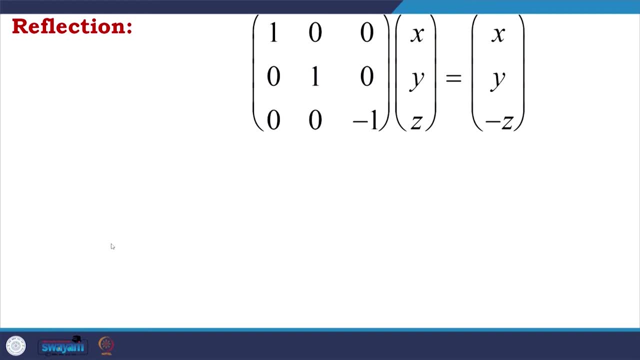 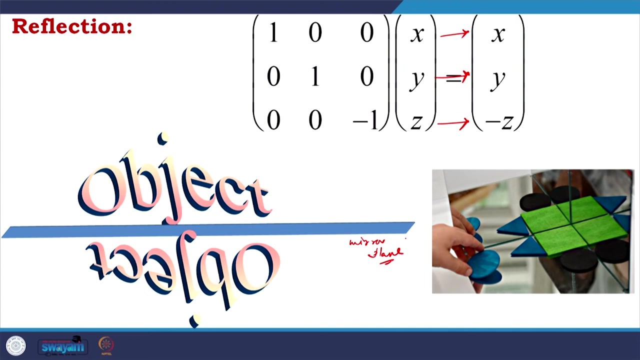 Coming to reflection, which is mirror. So it would be change from one axis: x return x, Y return y, and z goes to minus z. This is one of the representation. you see, the mirror plane, and this is a very beautiful representation. This is the mirror you see. Now see, if you. 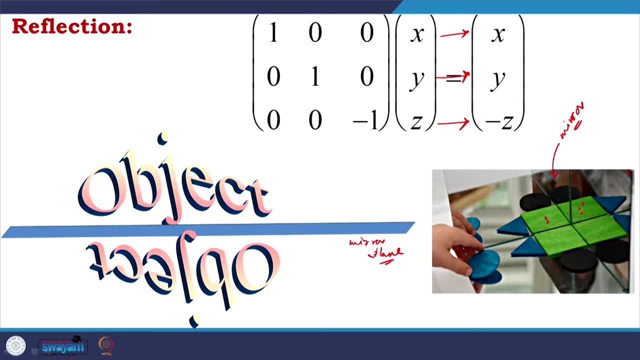 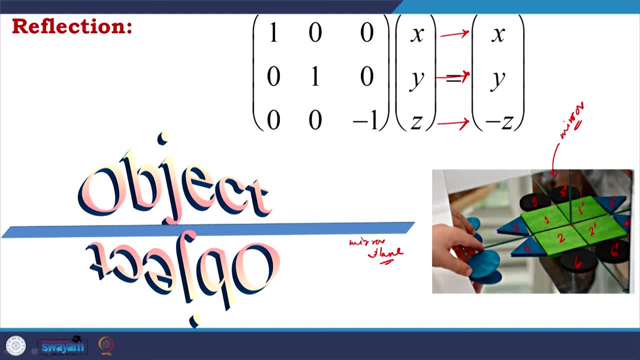 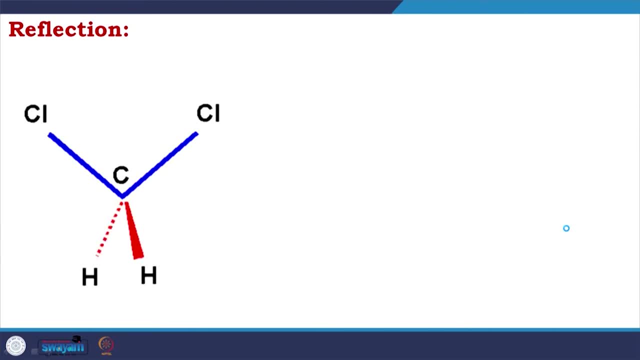 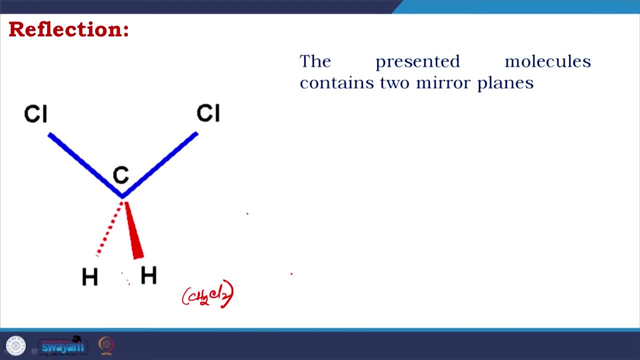 plane. See, if you have a symmetry like here, you will differentiate between this CCL and this CCL. but if you have it here, you differentiate CH with CH. So one is horizontal on the plane of the paper, bisects the CL, CCL bond or so. 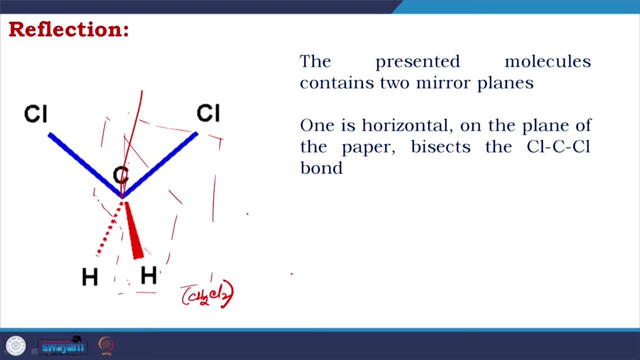 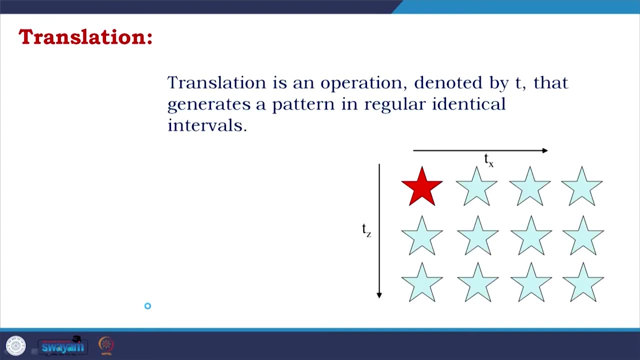 this is one so bisects like this. Other one is vertical, perpendicular to the plane of the paper. bisects HCH bond. Coming to translation, translation is an operation denoted by T that generates a pattern in regular identical intervals. So if you see, you go here. suppose this is the distance in the X axis, if I say X1 the 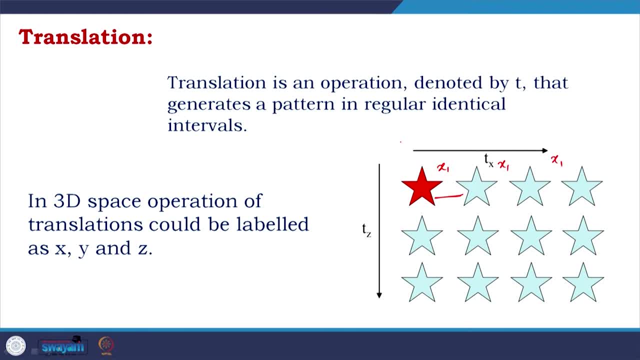 same distance in the crystal. So you go a translation of X and you generate one motif again, one motif, again one motif. If you go to Z, So this is 2D, but it could be 3D in a 3D space operation translation could be labeled. 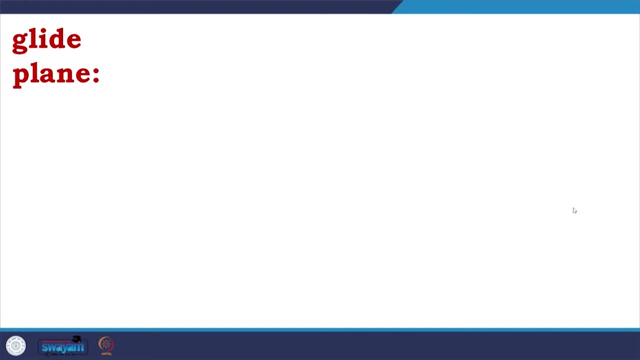 as XYZ. So you have 3 axis and their movement In the glide plane. this is interesting. you have one matrix and you have second matrix which tells you you have two operations leading leading to a result. So x is x plus half, y is y, z is minus z. So in the glide plane, 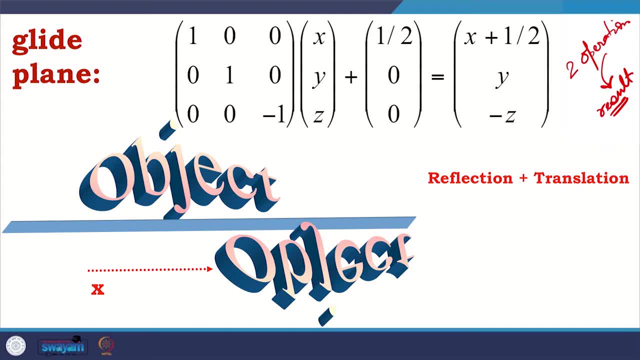 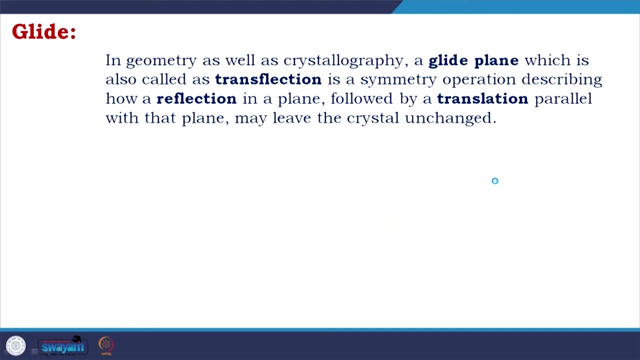 it is a combination of reflection along with translation: reflection in z axis and then half translation. So in geometry as well as in crystallography, a glide plane, which is also called as transflexion, is a symmetry operation describing how a reflection in a 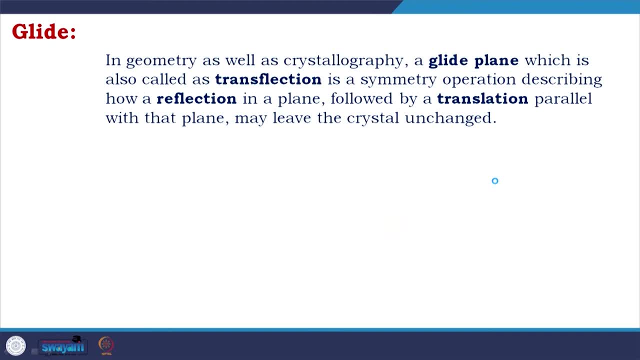 plane, followed by a translation parallel with that plane, may leave the crystal unchanged. A very good example. A very good example is this, where you see that here there is a reflection. if you put a mirror you will have a reflection, but with the reflection would be putting the feet here. 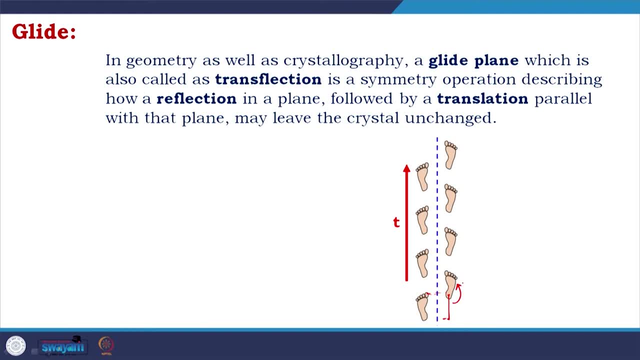 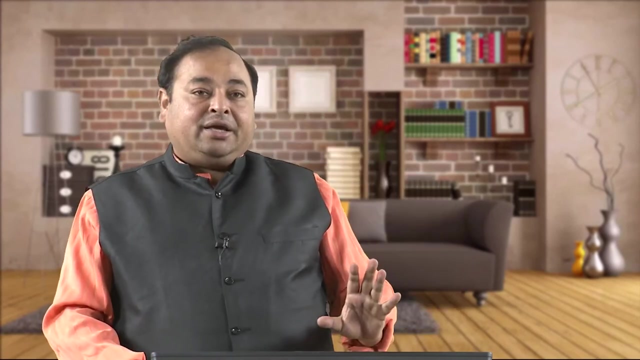 but the feet is now proceeded. So there is a reflection followed by a reflection which, by a translation, a two step operation: reflection followed by translation. Example of glide. you see, and one of the very beautiful natural example of glide you will see, when you go to any beach, you will see people walk generally, when people walk, they 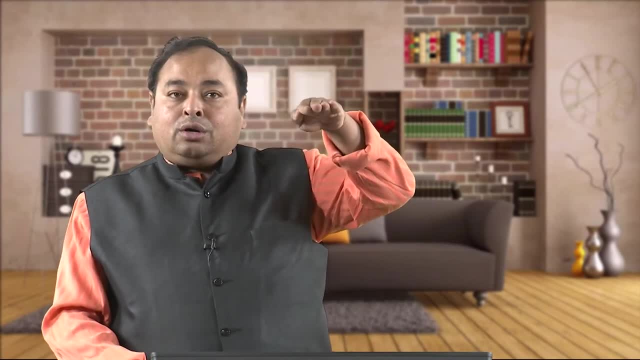 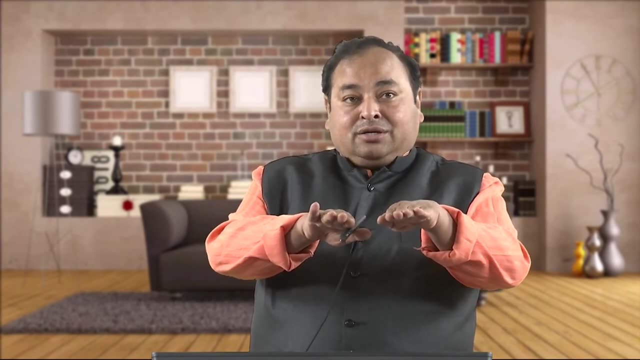 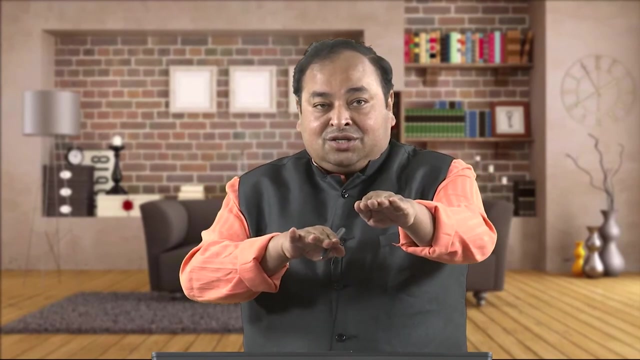 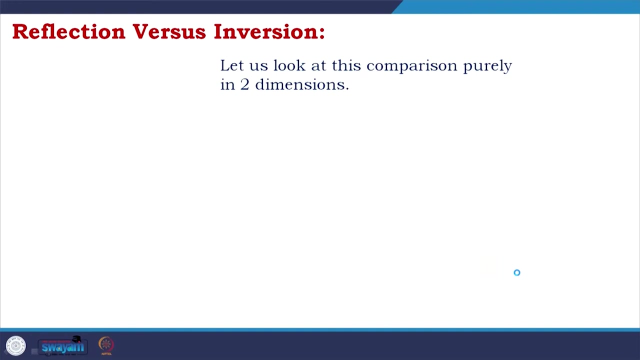 follow glide motion because you have your one feet. the other feet is a mirror plane, but so it is a reflection, but it always proceed. So you have your first feet, your second feet Going ahead. that is called glide. Let us take a comparison to understand reflection and inversion. 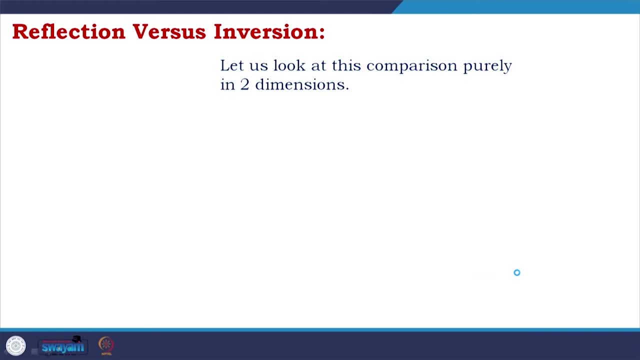 For that, let us look at this comparison: fuel in two dimensions. first, Reflection of a two dimension object occurs across a plane mirror. So you see, this is a reflection. So here this point and this point are in equidistance, as well as this point to this point, but this: 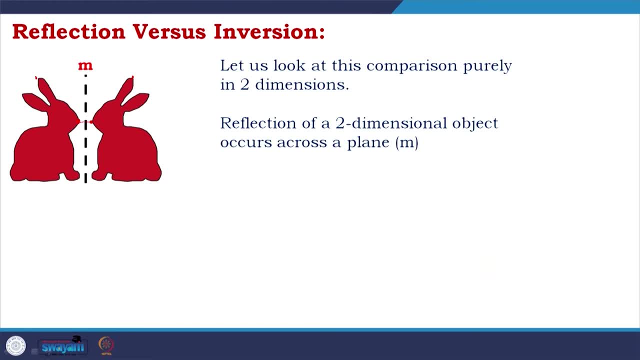 equidistance would be going through this, whereas so the equidistance would be measured from the mirror axis A, B, A always equal to B, so as A prime, B, prime After inversion, everything is an equivalent opposite distance through a single point, i. So, if you see, this is the. 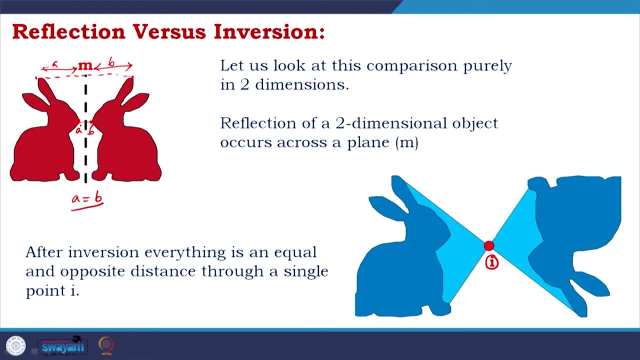 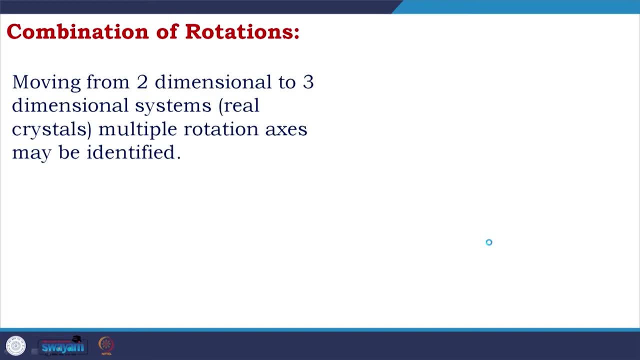 point of inversion, you get those equidistance like you get here, but here through this point, only here, through this axis, that is the difference. Now we will discuss the combination of rotations. so, moving from 2 dimension to 3 dimension, which are the real system, multiple rotation axis may be identified. 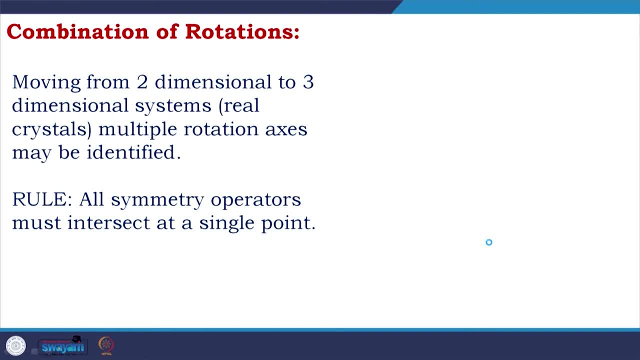 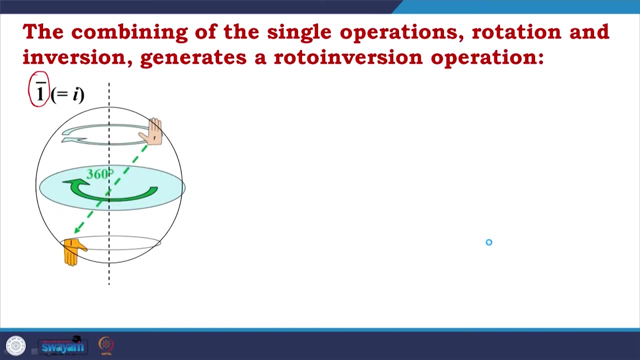 The rule is all symmetry operators must intersect at a single point. So you have the rotations 2 fold, 3 fold, 4 fold, 6 fold, but along with that you should have the mirror plane. The combining of single operation, rotation and inversion generates a roto inversion operation. 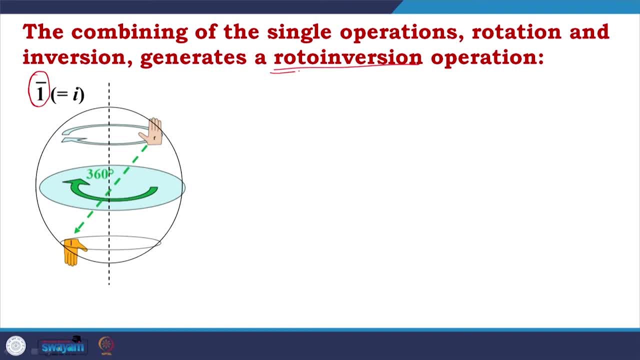 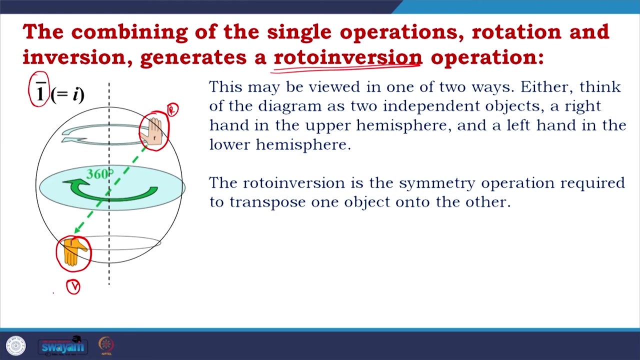 this is a 3 dimensional operation. So you have this picture. if you think of the diagram as to independent object, you have a right hand in the upper hemisphere and you have a left hand in the lower hemisphere. So you have a right hand and you have a left hand. the roto inversion is the symmetry operation. 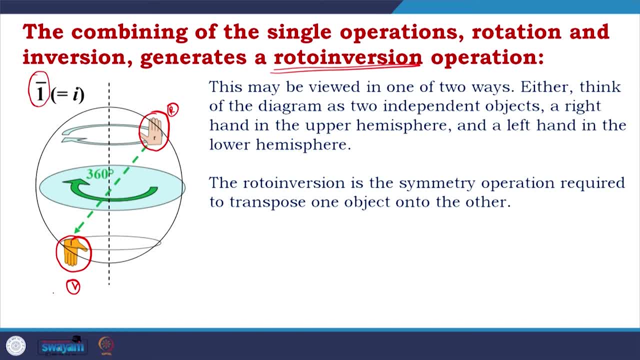 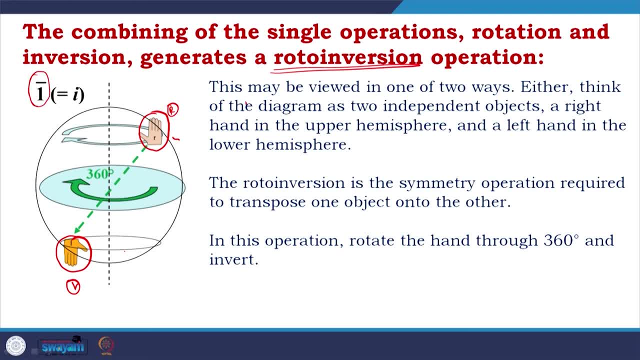 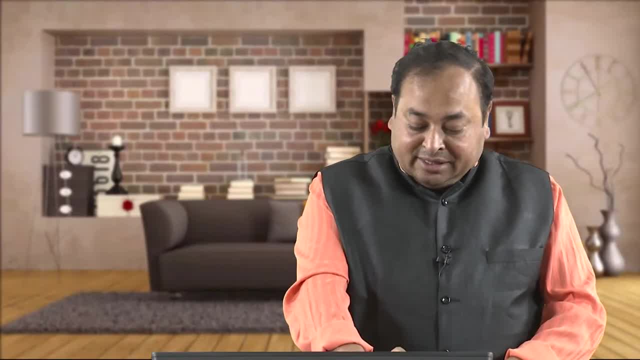 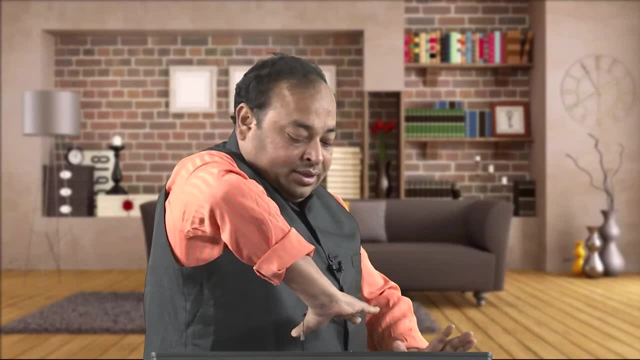 So you rotate the hand from here to 360 degree and then you invert that, So you have this, you do that and you invert, so you get like this, So you have like this, and then you do that 360 and then invert. you will see that it would. 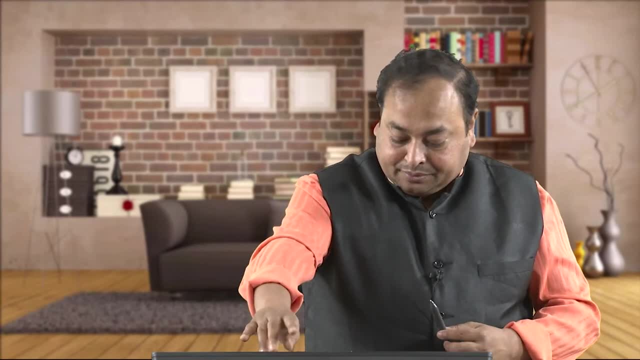 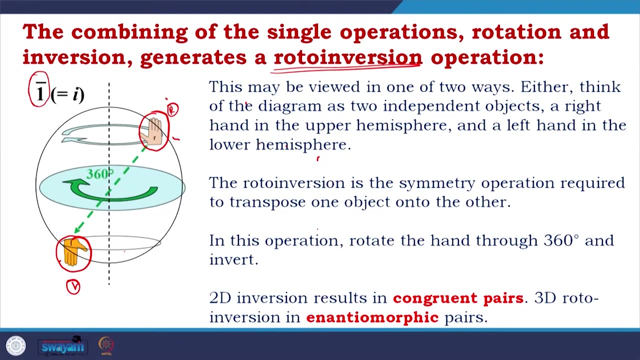 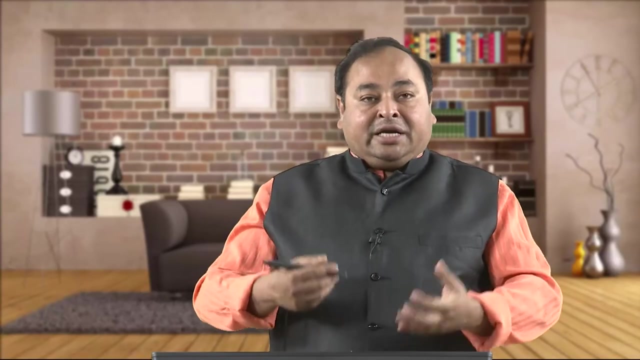 be like this: 2D inversion results in congruent pairs, whereas 3D- roto inversion- in enantiomorphic pairs. Remember, I did not talk about the congruent pair, but I told when the time will come. Now it is a time when we are converting our self from 2D to 3D, because we always do 2D. 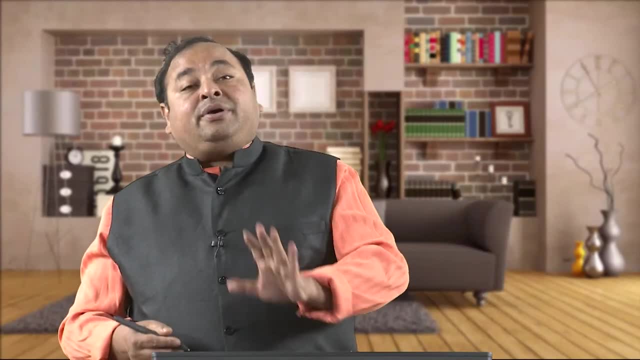 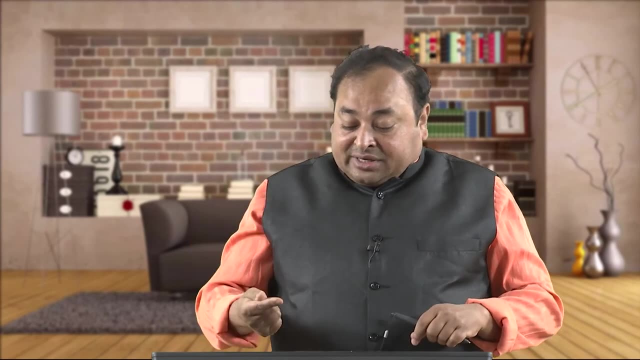 because 2D is easy to understand but we have to do 3D because 3D is actual, real system. So in 2D inversion results congruent. So in 2D inversion results congruent. So in 2D inversion results congruent. 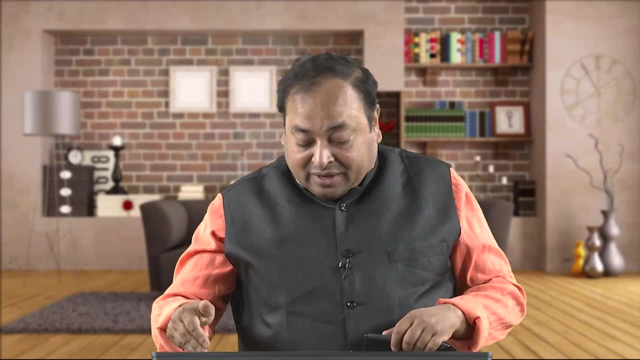 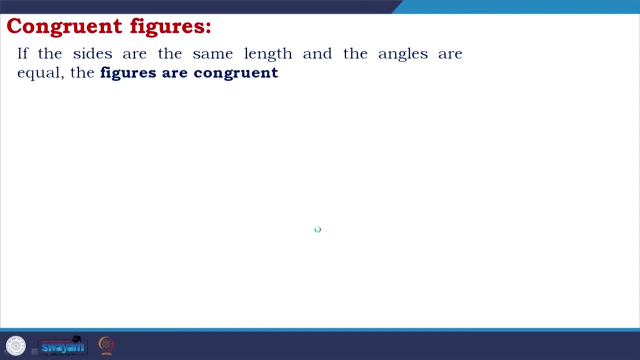 So what are they For? a congruent figure or congruent pair: if the sides are the same length and the angles are equal, then the figures are called congruent. Each side, an angle of one figure, correspond to a side, or angle to the other. we call this. 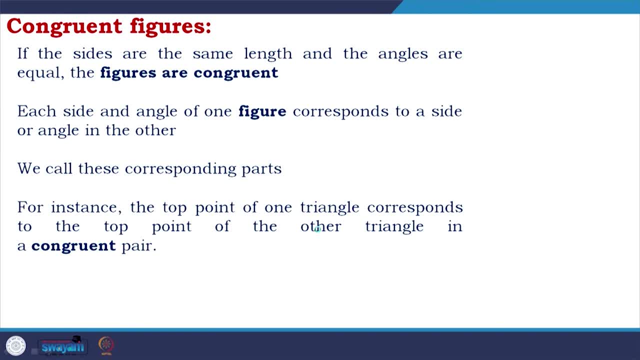 these corresponding parts. For an example, the top point of one triangle correspond to the top point of the other triangle in a congruent pair like this, but it could be in different form, like this also. So this is also a congruent pair, and even when they are not having a regular shape in 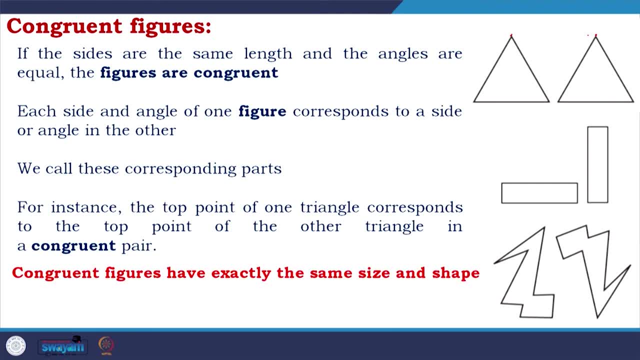 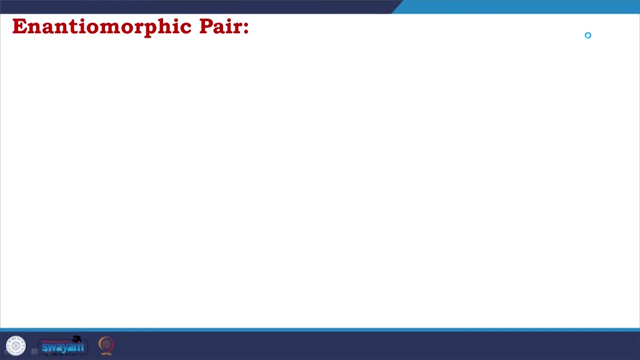 that time also, they could be congruent pair. So congruent figures or congruent pair have exactly the same size and shape, They have congruent sides and congruent angle. Now what is enantiomorphic figure or enantiomorphic pair? Pair of compounds, crystal molecules that are mirror images on each other but are not congruent. 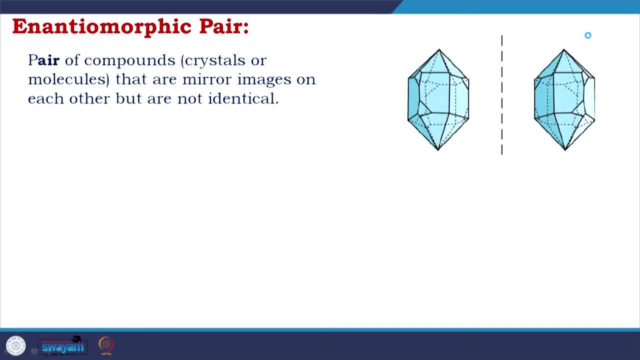 Not identical So you could see the pair of crystals. they are enantiomorphic pair. So we talked about in the 2D inversion results in congruent pair. 3D roto inversion in enantiomorphic pairs. So we already talked about. now you could put this on top of this, but now you understand. 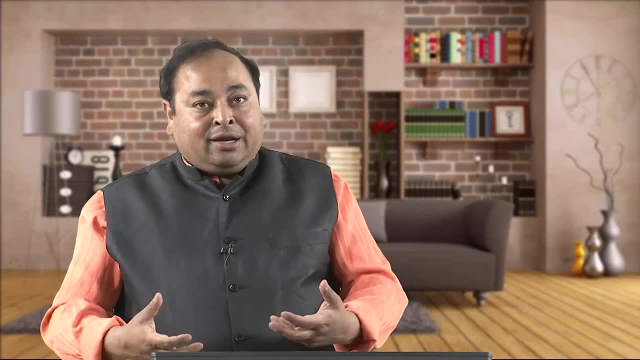 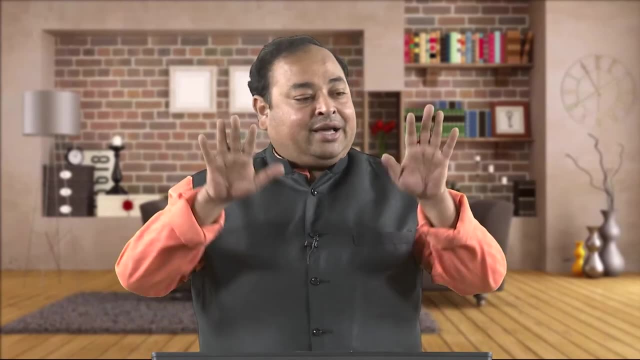 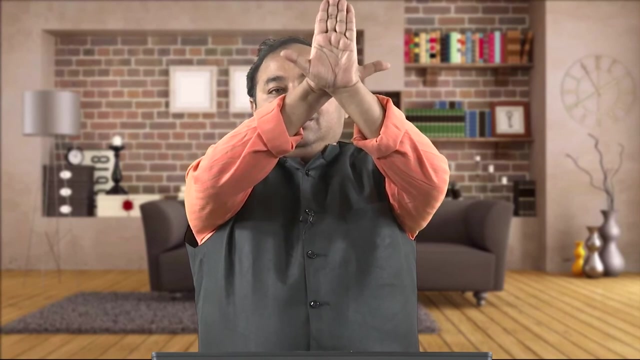 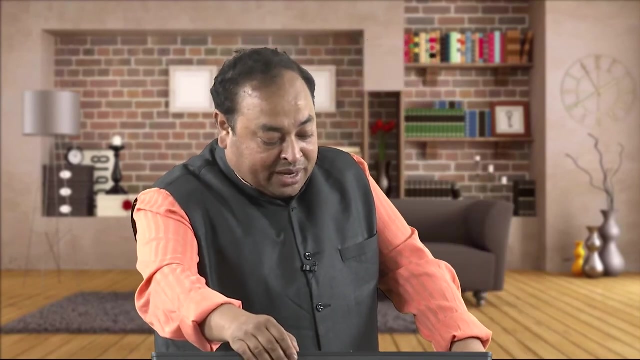 we have already shown you in the model That this is a chiral pair and they are not superimposed like hands. if you want to put them on the top of each other, these two would not be superimposed. So that is the difference between a congruent pair and a enantiomorphic pair. 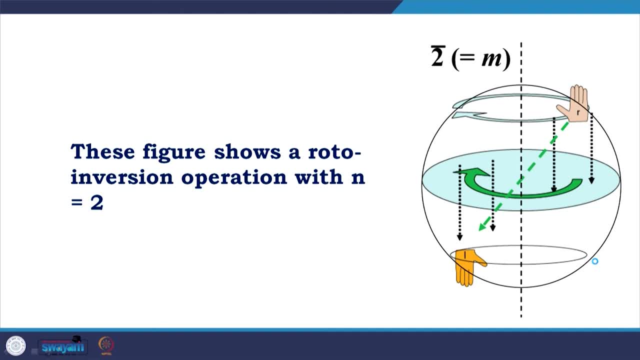 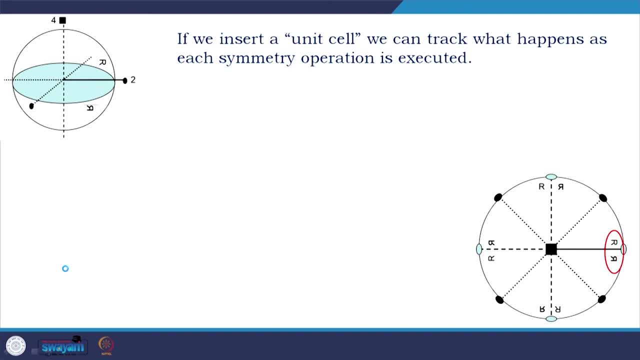 we can track that what happens as each symmetry operation is executed. So we are putting a unit cell. viewing the image from above means on the top 4 fold axis, which is 90 degree, 4 fold rotation of the original R motif results in the way we will see the change in the figure. 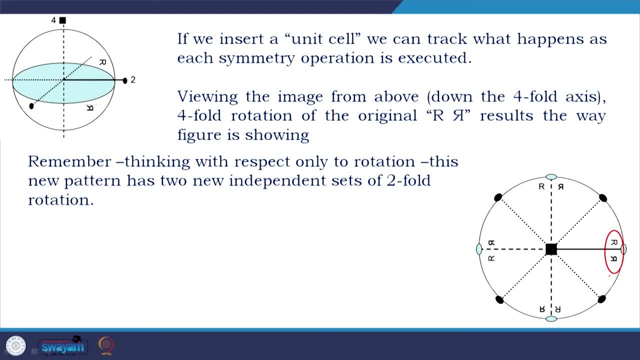 Now remember thinking with respect only to rotation. this new pattern has 2 new independent sets of 2 fold rotations: The first one we have highlighted and, like this, and this set themselves generate the second set of 2 fold rotation which is indicated by the black marker. 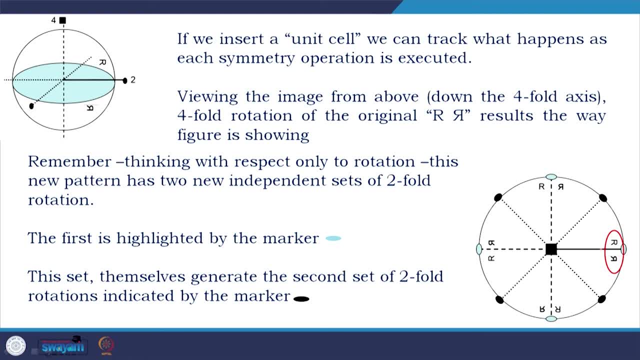 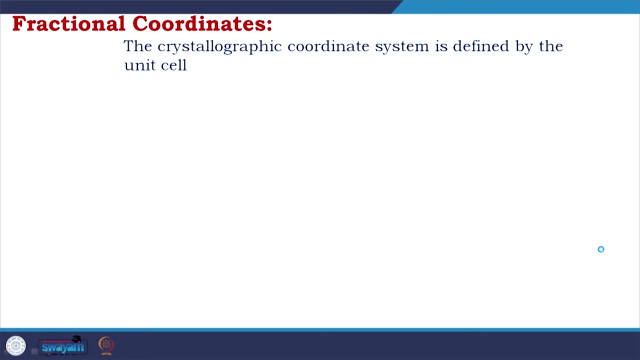 So we start from here, then we have created- initially We get a new pattern, and then this new pattern generate itself the second set of 2 fold rotations. here I talk about fractional coordinates. The crystallographic coordinate system is defined by unit cell. The location of a point is defined by fraction of travelled from 0. 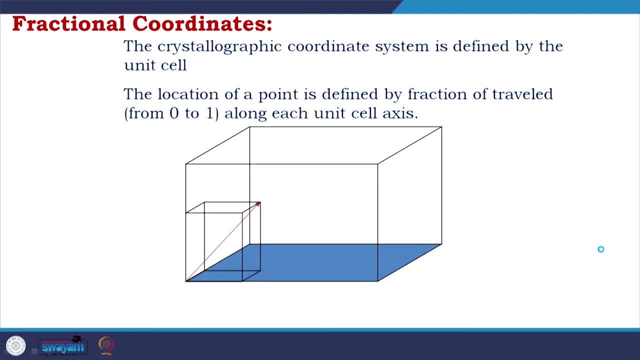 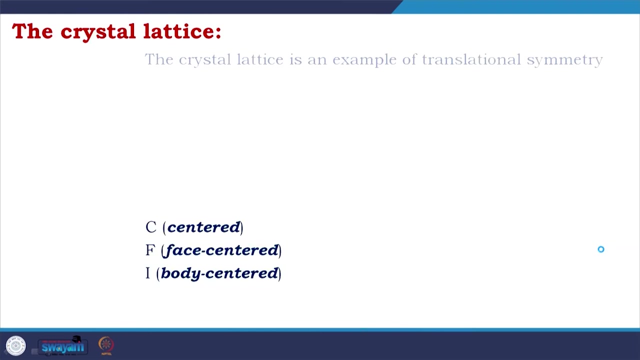 to 1 along each unit cell axis, which we have talked about about. but let us say here we have a fractional axis: 0.33, 0.25, 0.55, so the fractional coordinates are always measured parallel to each axis. the axis are not necessarily 90 degree apart. 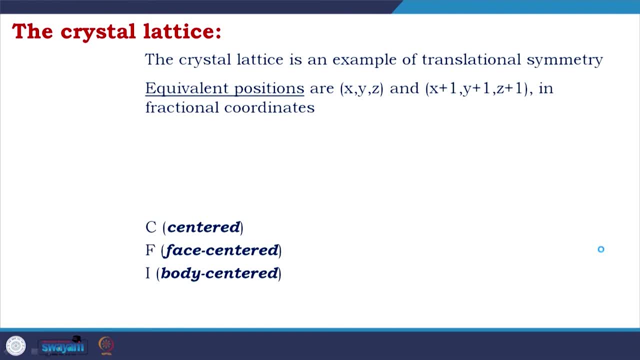 The crystal lattice is an example of translational symmetry. equivalent positions are x, y, z plus 1, x plus 1, y plus 1, z plus 1, so one translation in fractional coordinates. Space groups that have no other translational symmetry operations are called primitive space. 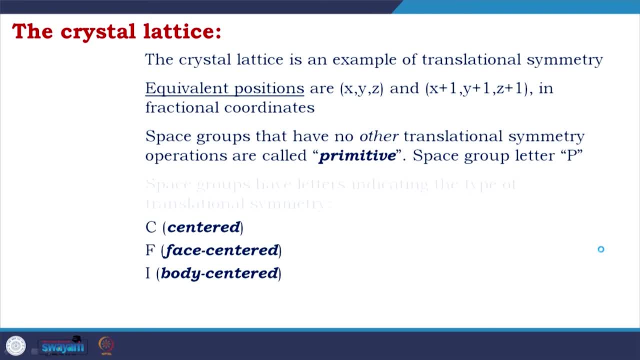 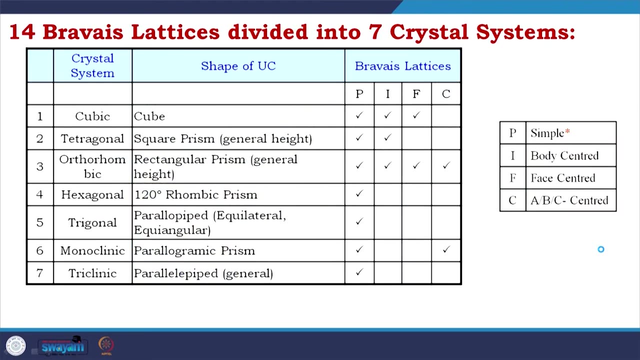 group and represent with a letter P but space group have letters indicating the type of translational symmetry: S centered, so center base translation F, F centered and I body centered. And all those gives rise to 14 revised lattices which are divided into 7 crystal systems. 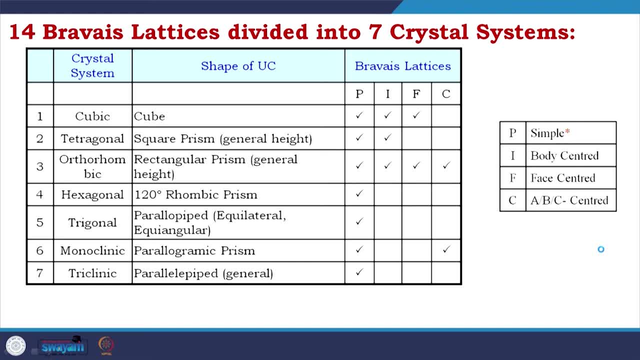 So the 7 crystal systems are cubic, tetragonal, orthorhombic, hexagonal, trigonal, monoclinic and triclinic. The cubic crystals have the shape of cube, Tetragonal have the shape of square prism, orthorhombic, rectangular prism, hexagonal. 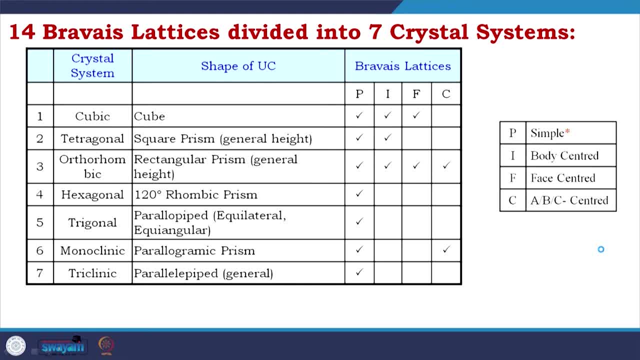 120 degree rhombic prism, trigonal parallelepiped, monoclinic parallelogramic prism and triclinic parallelepiped From this 7 crystal system. who are the 14 revised lattices for cubic? there are 3 for 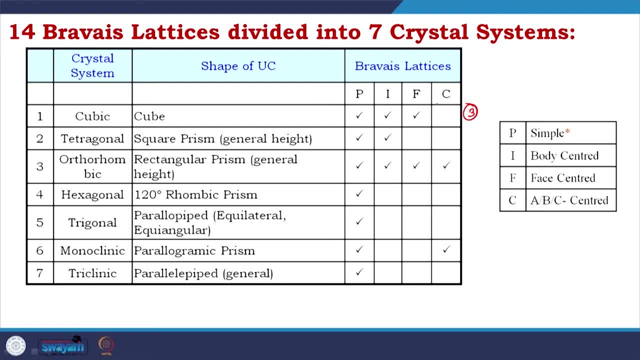 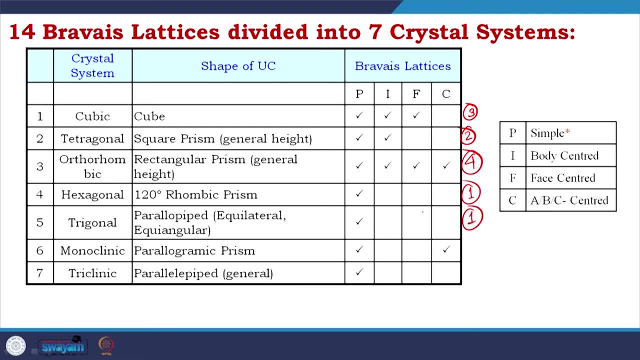 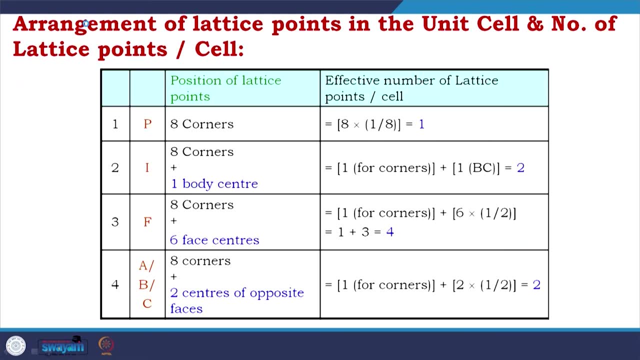 So 14 revised lattices divide into 7 crystal system. Arrangements are for 4, hexagonal 1, trigonal 1, monoclinic 2, triclinic 1.. So 14 revised lattices divide into 7 crystal system. 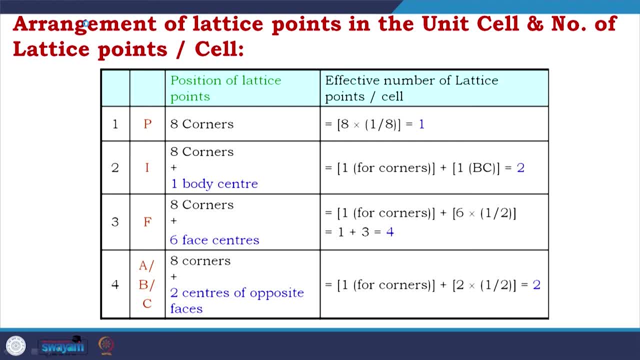 Arrangements are for: 3. For tetragonal 3, hexagonal: 1.. arrangement of lattice points in the unit cell and number of lattice points per cell. So if it is primitive there are 8 corners and effective number of lattice points per. 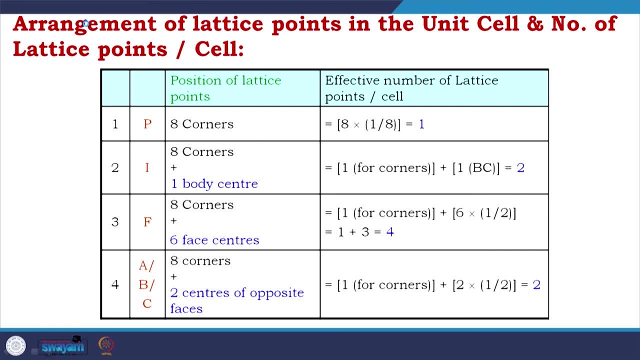 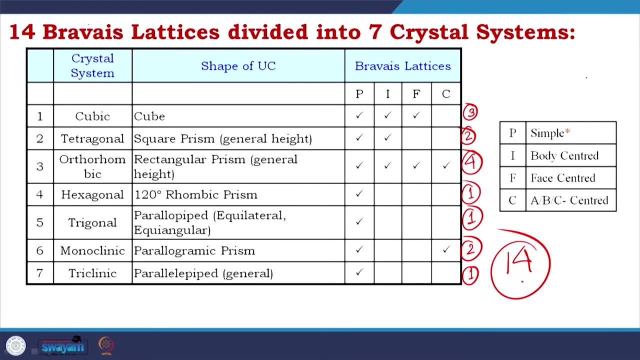 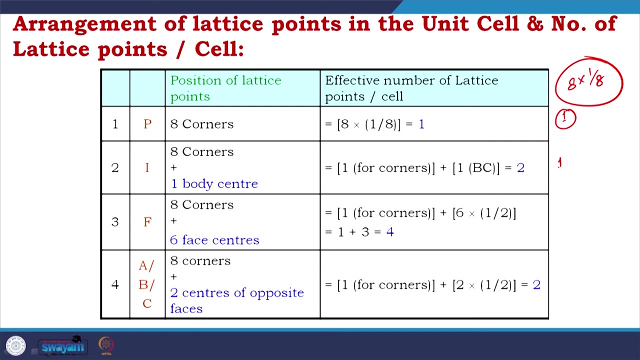 cell is 8 into 1 by 8, 8 points, so 1, 8 into 1 by 8.. For I, if you do not remember, go back I- is body center, center at the body, so 8 corner and 1 point for 1 body center. so 1 plus 1 is 2.. 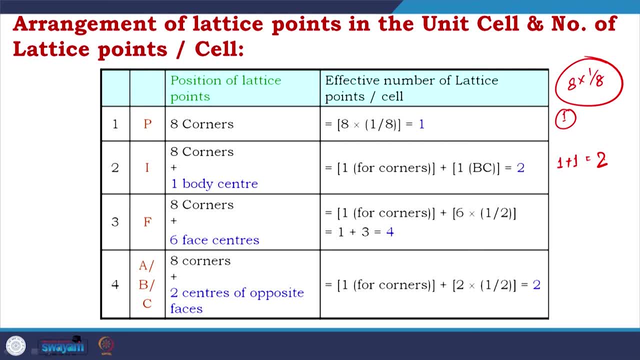 For F it have faces, so 6 face and 8 corners. so 1 plus 1 is 2.. 3 equal to 4. and then for the C centered A, B, C, so it have 2 centers of opposite faces. so 1 for corners everyone is having, and then 2 into half because it is either A or B or 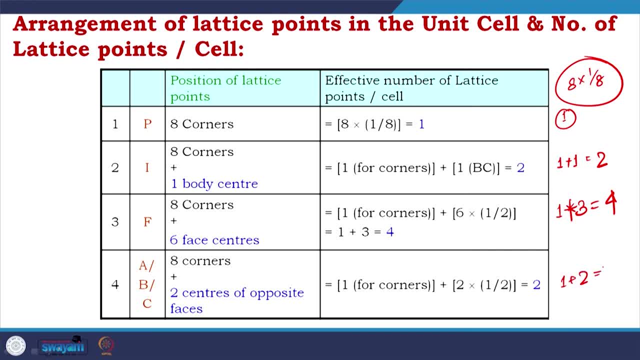 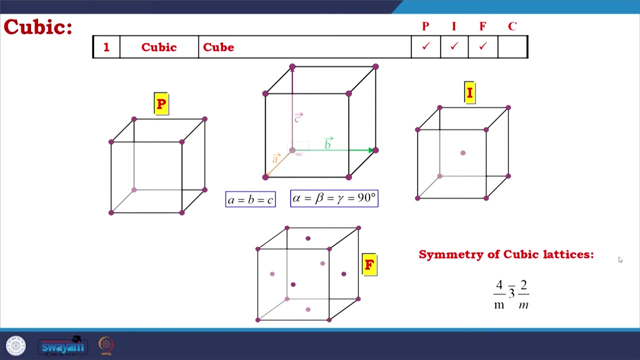 C. so 1 plus 2 is 3.. Sorry, 1 plus 2 into half, because you have the centers of opposite faces. so contribution of half 2.. Now looking at the details of the 7 crystal system, what we talked about. so here in the 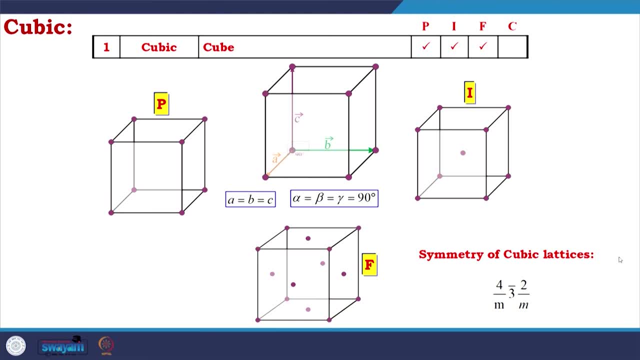 cube. it have primitive body centered face centers. the conditions are A equal to B equal to C and alpha equal to beta, equal to gamma equal to beta. It has a symmetry of 90 degree, so its perfect shape. the symmetry operations are 4 by m 3. 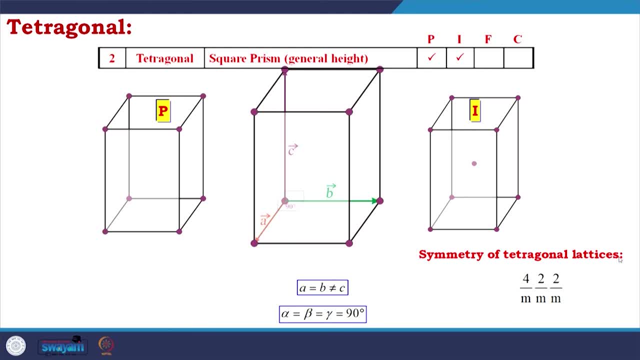 bar and 2 by m. Tetragonal: for tetragonal there is primitive and body centered. so here, A equal to B, not equal to C, alpha equal to beta, equal to gamma, equal to 90 degree. symmetry: 4 by m, 2 by m. 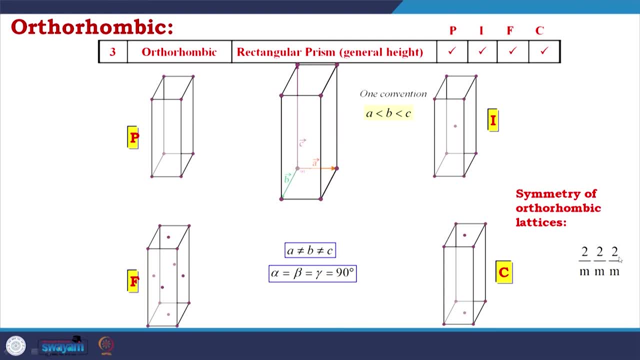 2 by m, So this is the perfect shape. the symmetry operations are 4 by m, 3 bar and 2 by m, So it is a perfect shape. Orthorhombic. it have all the contributions: primitive, body centred, face centred, C centred. 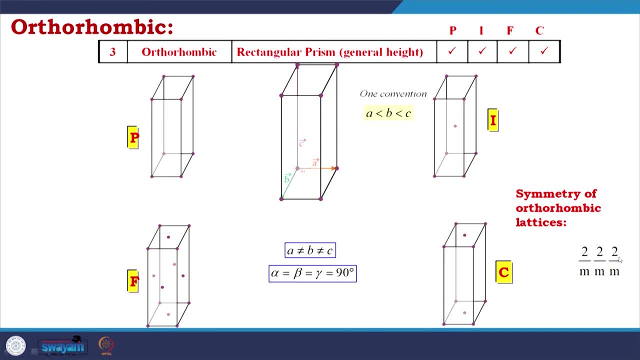 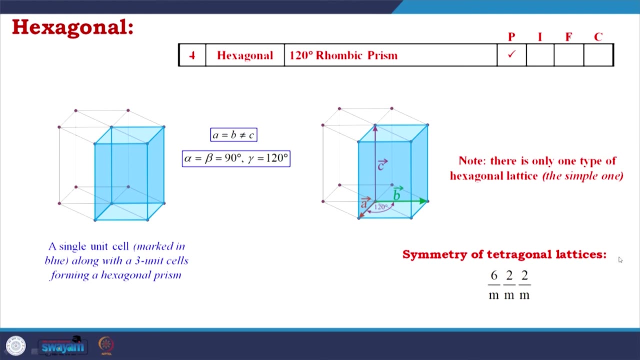 A not equal to B, not equal to C. the hands, the basis: angle alpha equal to beta equal to gamma equal to 90 degree. symmetry: 2 by m, 2 by m, 2 by m, hexagonal. you will note that here only primitive for the hands: A equal to B, not equal to C. angles alpha equal to 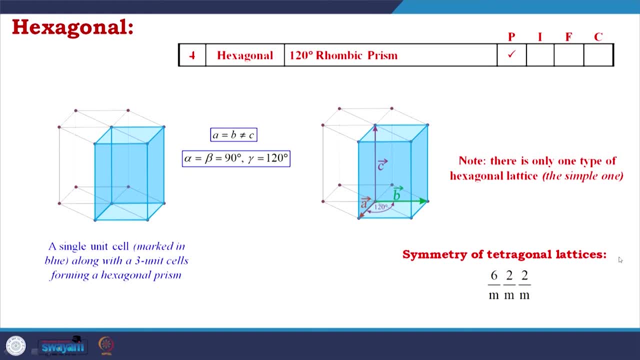 beta equal to 90 degree, gamma equal to 120 degree. As I told, there is only one type of hexagonal lattice: the simple, the primitive one: a single unit cell marked in blue, along with a 3 unit cell forming a hexagonal prism, if you see. 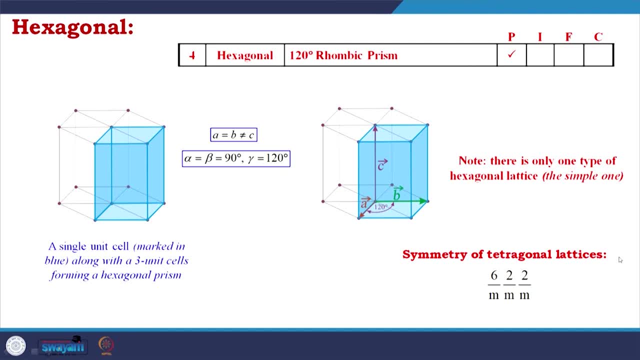 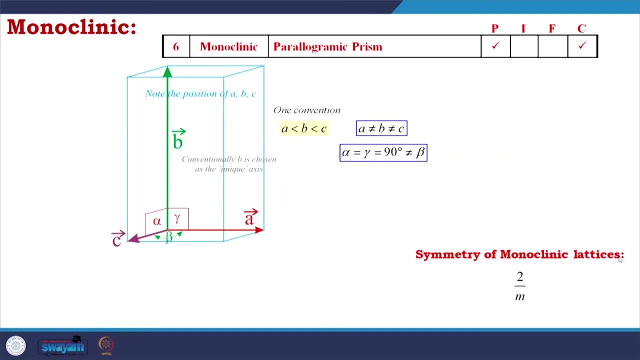 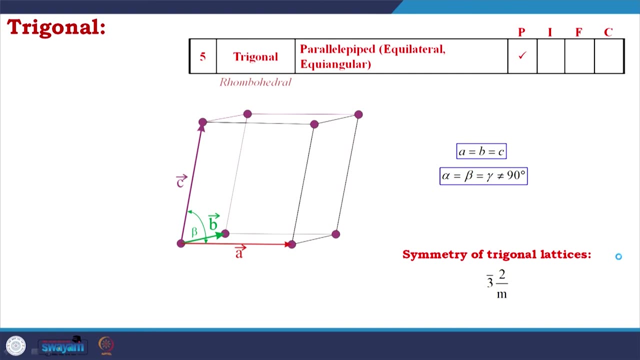 The symmetry 6 by m, 2 by m, 2 by m, 2 by m, trigonal. it could also called as rhombohedral. it have only primitive again: A in case of trigonal, A equal to B, equal to C, alpha equal to beta, equal to gamma, not. 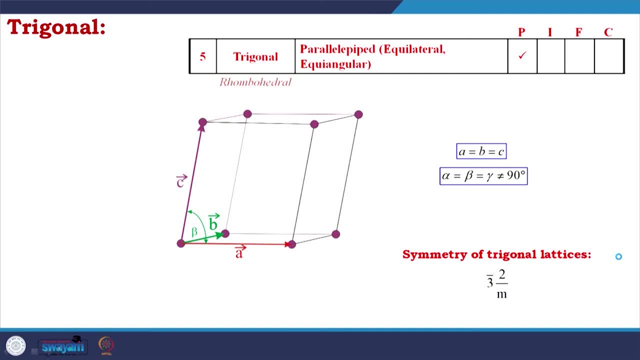 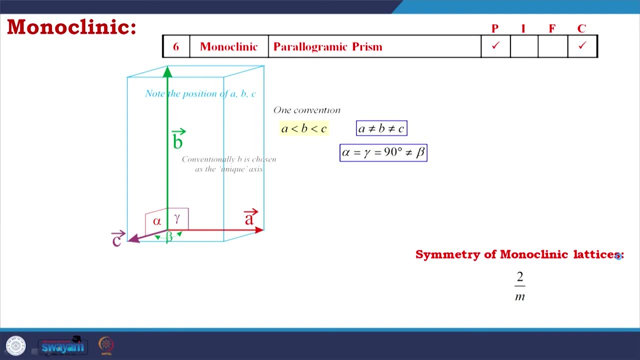 equal to 90 degree. symmetry 3 bar 2 by m, monoclinic primitive and C centred here. A not equal to B, not equal to C. For the Sides n: A less than B less than C. alpha equal to gamma, equal to 90 degree, not equal to beta. 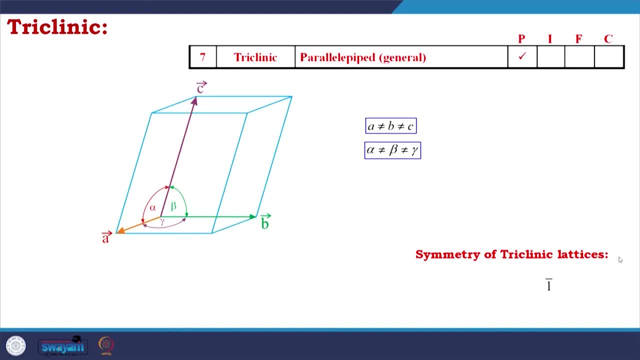 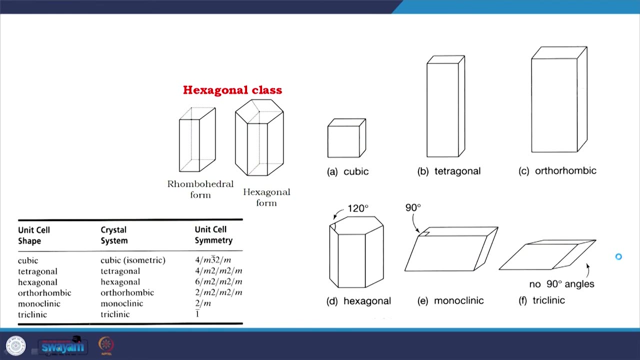 the symmetry is 2 by m, only triclinic. it is primitive, A not equal to B, not equal to C, alpha not equal to beta, not equal to gamma. it only 1 bar is the symmetry operation. So, as I told, unique cells. 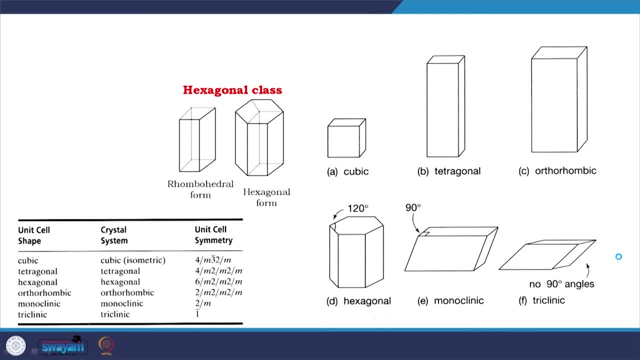 Shape- cubic tetragonal, hexagonal, orthorhombic, monoclinic and triclinic crystal system. according to cubic, tetragonal, hexagonal, orthorhombic, monoclinic and triclinic. Here you see 6, but we have 7 because hexagonal class of 2, the rhombohedral form and the hexagonal 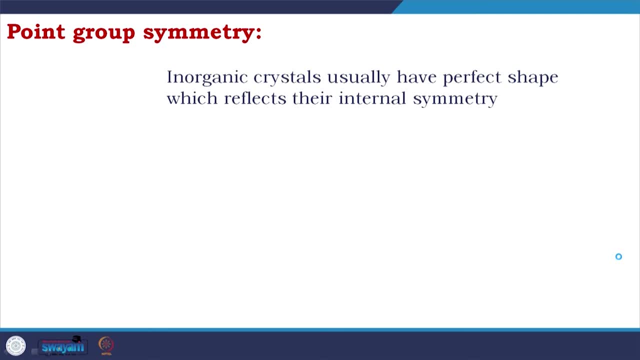 form. the point group symmetry in the inorganic crystal. Usually they have perfect symmetry. So the point group symmetry in the inorganic crystal. usually they have perfect symmetry. This is lecture which we will be interested. inarde anina word And in the next lecture I will give analysis further on in졌, which reflects in the internal. 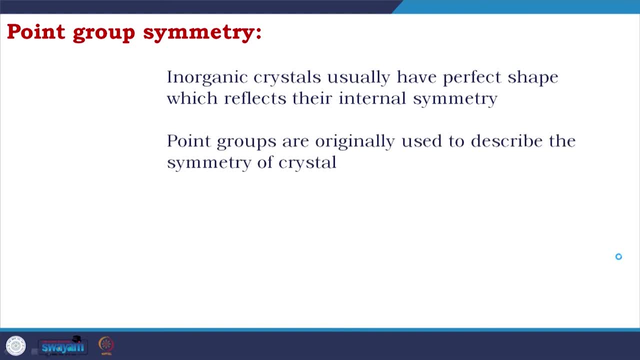 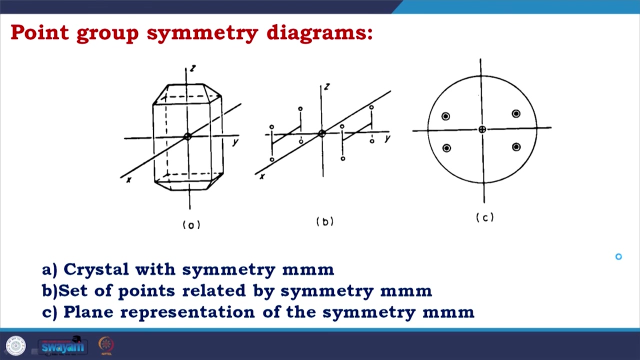 symmetry point groups are originally used to describe the symmetry of crystals. point group symmetry does not consider translation and included symmetry elements are rotation, mirror plane, center of symmetry and Roto inversion. So when you see crystal with symmetry M, M, M, M, M, the mirror plane set of points related by symmetry M, M, M and plane represented for 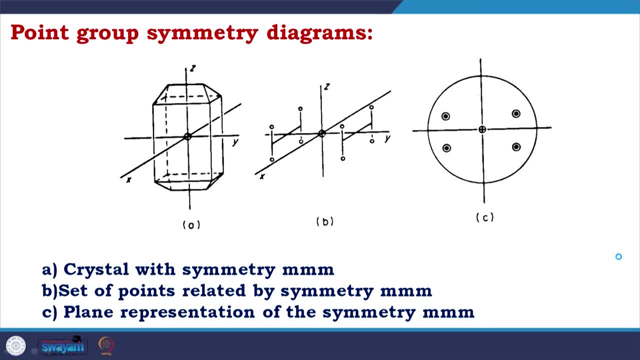 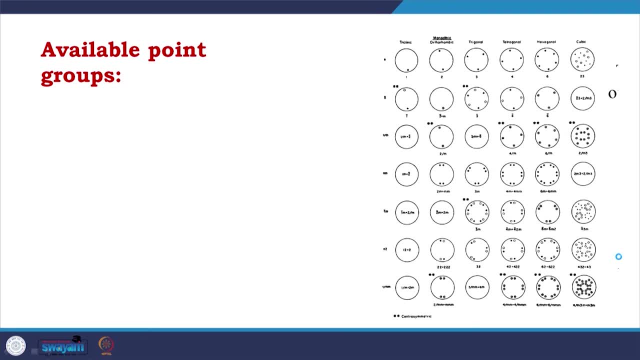 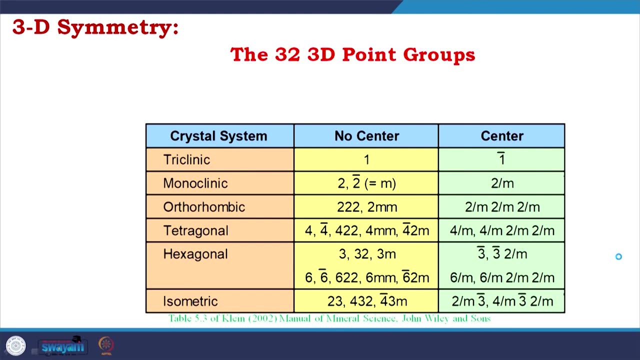 the symmetry M, M, M, the mirror. So point group symmetry diagrams. these are the available point groups. not going into details, I rather come into the 3D symmetry. We have 32 3D point groups. it regroup by the crystal system and it have consideration. 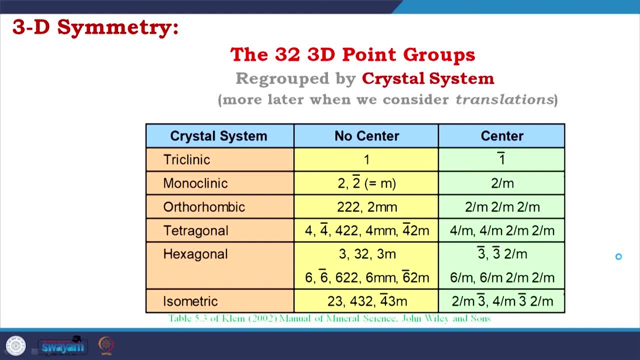 no centre and it have consideration of centre, which is the consideration of translation For triclinic: no centre, it is 1 centre, it is 1 bar. monoclinic: 2, 2 bar and 2 by M orthorhombic: 2, 2, 2, 2 M M. 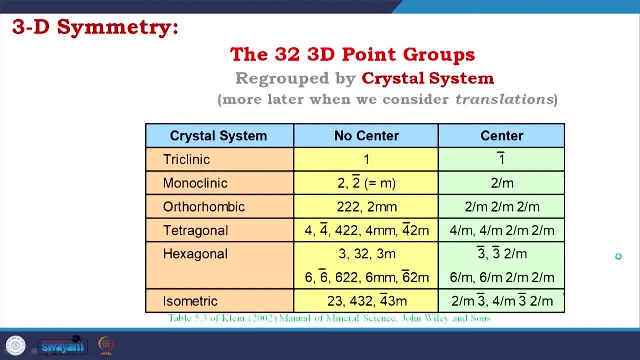 With centre 2 by M 2 by M 2 by M tetragonal 4, 4 bar 4, 2, 2, 4 M M, 4, bar 2, M. with centre 4 by M 4 by M 2, by M 2 by M. hexagonal 3, 3, 2, 3, M, 6, 6 bar 6, 2, 2, 6 M M, 6, bar 2 M, 3, bar 3. 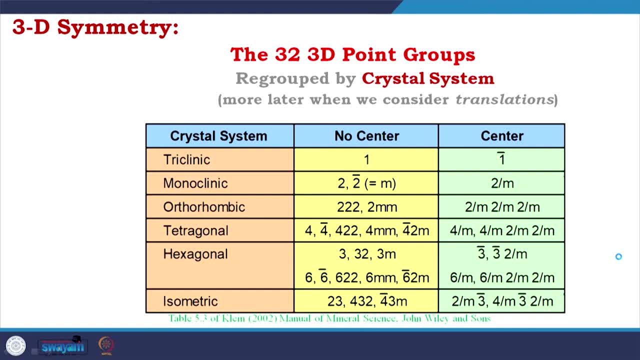 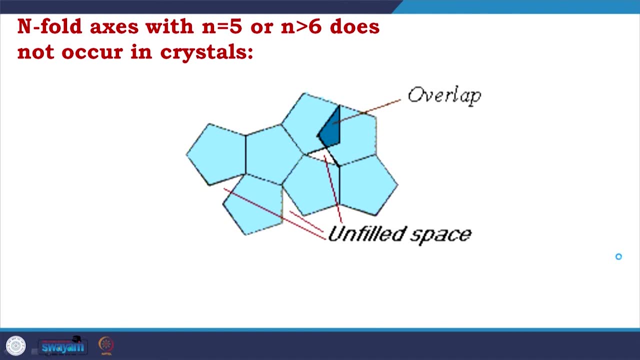 bar 2 by M, 6 by M, 6 by M, 2, by M, 2 by M, Isometric 23 432. 3 by M, 3 by M, 3 by M. I talked about n fold axis where n equal to 5 or n greater than 6, they does not occur. 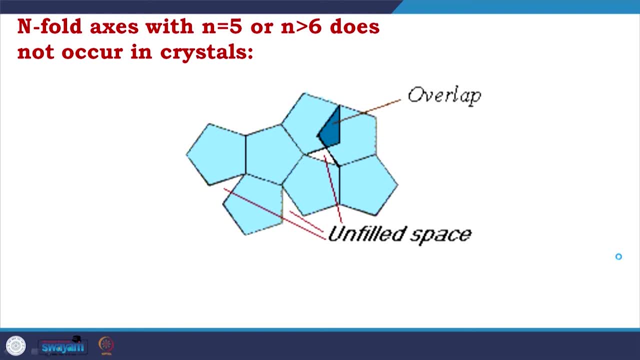 in the crystal, because in those cases there are overlaps, there are unfilled space, which are not favorable for the formation of the crystals. So the adsorption spaces must be completely filled, So the adjarection spaces must be completely filled. So the adjarection spaces must be. 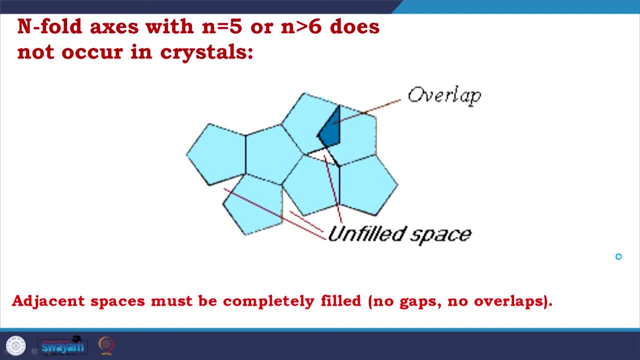 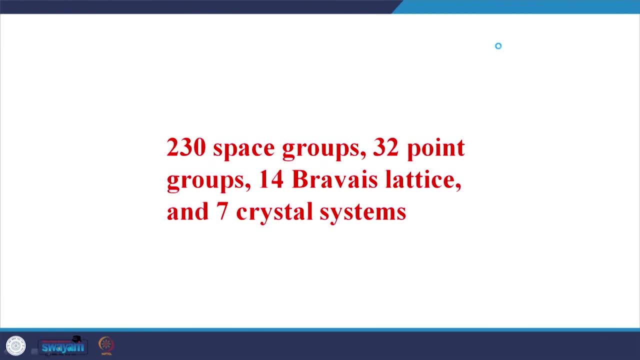 to get perfect symmetry which comes in the n equal to 2, n equal to 3, n equal to 4 and n equal to 6.. Overall, there are 230 space groups, 32 point groups, 14 Bravais, lattice and 7 crystal systems. 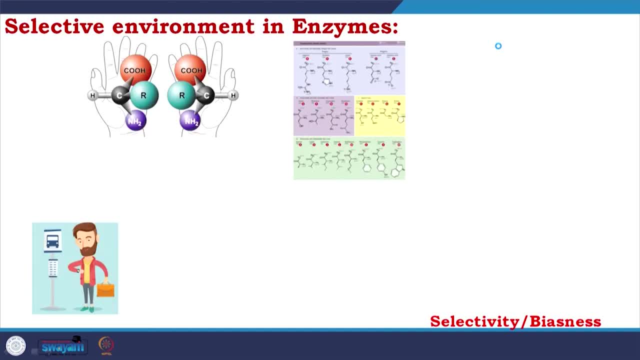 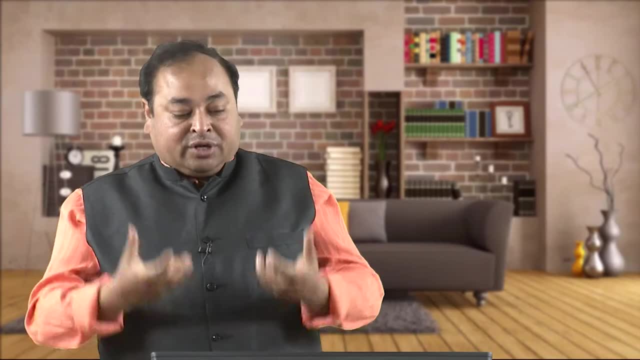 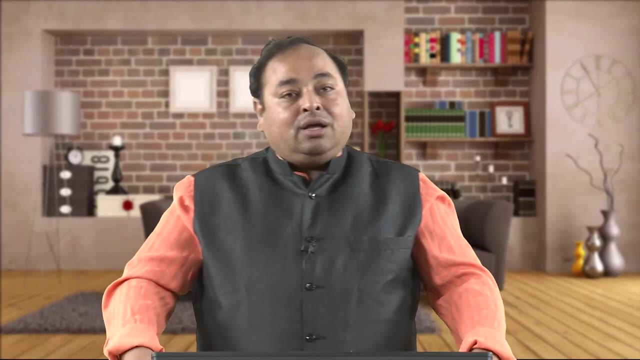 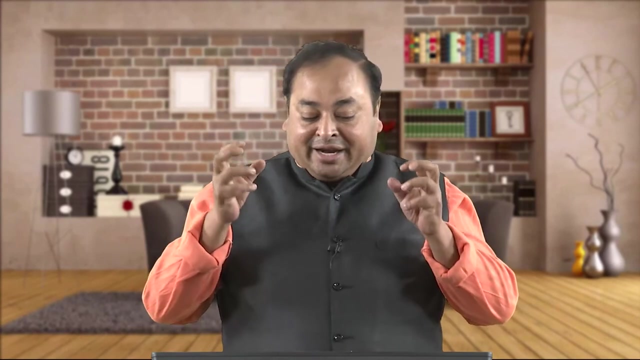 which we are discussed. But now we have to talk about selective environment in enzymes or proteins, which is our focus. We already talked about chirality. we talked about the amino acids. the amino acids maintain chirality, So you cannot get D amino acids, you only get L amino acids. 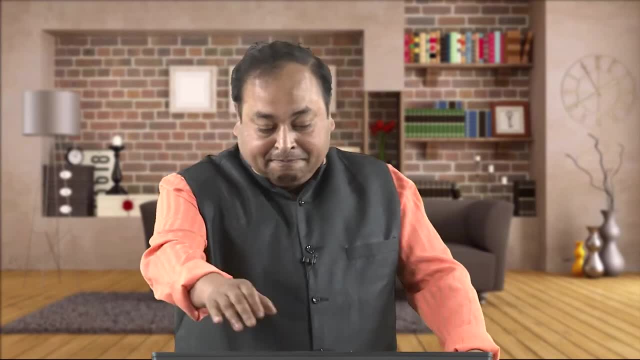 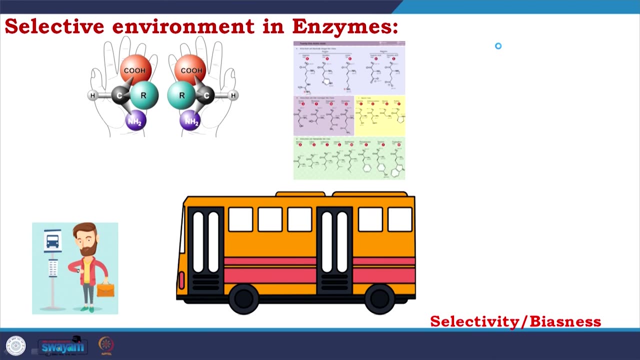 Here I am going to talk about an interesting story. So you look at this person who is C Standing or waiting at the bus stop. The bus appears. the bus have two doors. you could say front door and back door. The guy could avail both the doors. it have equal chance. 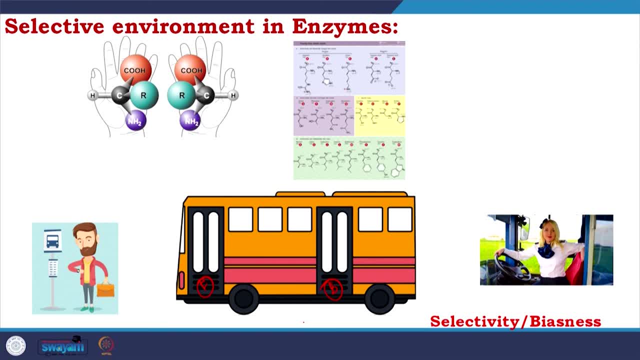 Now, suddenly, the guy have observed the driver. there is a beautiful driver, So now the equivalent of the driver. the driver is standing or waiting at the bus stop. Now, suddenly, the guy have observed the driver. there is a beautiful driver, So he must have a valid chances of front door and back door. 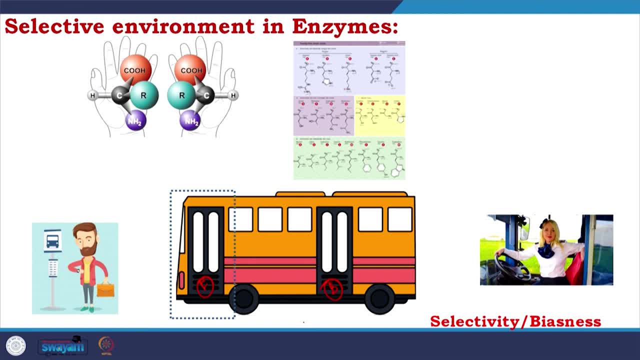 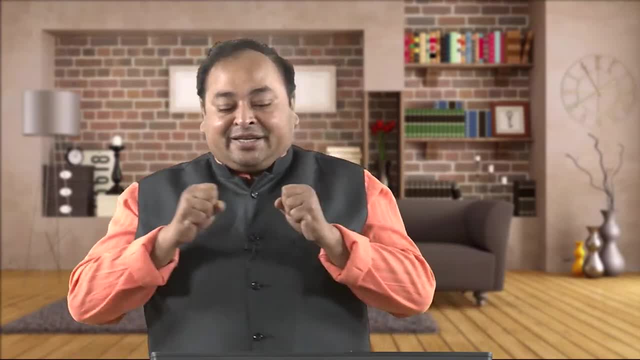 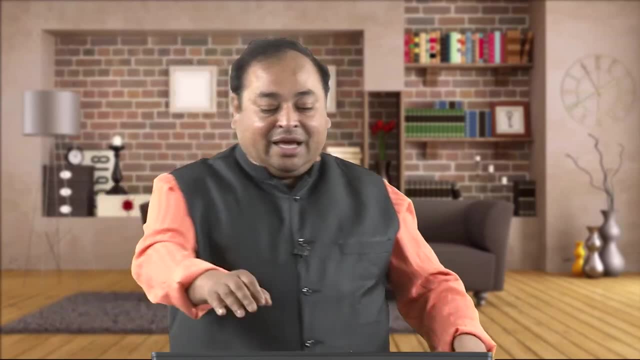 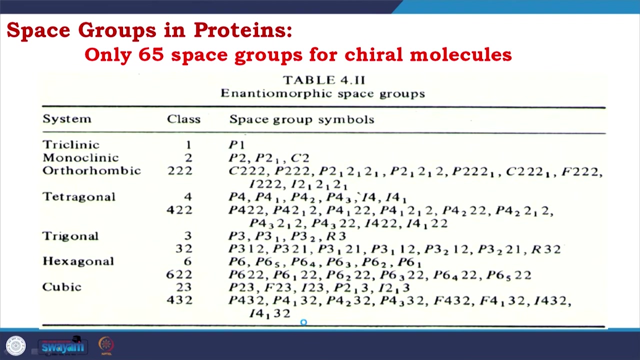 To him, the preference become front door. Similarly, in enzyme or protein, specially in enzyme, when it goes for the catalytic reaction, the choice becomes depending on the chiral environment and also when you are considering here, As I told, the recent research. 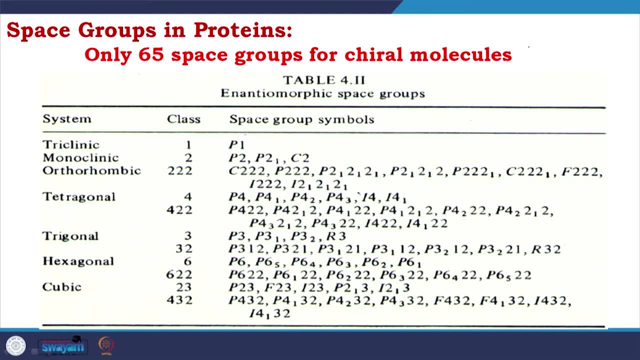 Lecture 6.. 230 space group. it reduced to 65 for protein because of its chiral environment. So we have talked about the basic symmetry, we have talked about how those symmetries are operated using matrix operation. we have talked about the importance of those symmetries. 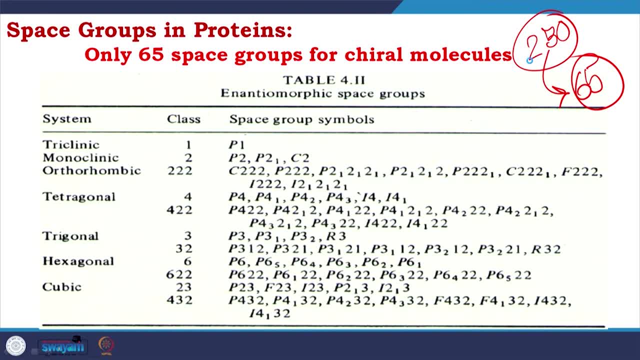 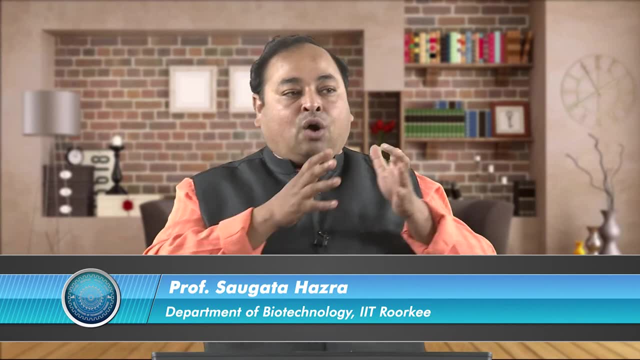 especially when they are in 2D. we understand well, but when it comes to combination it is relatively difficult to understand. but they are the one which are actually present here. So we talked about the combination, we talked about the operation, how that gives to a system. 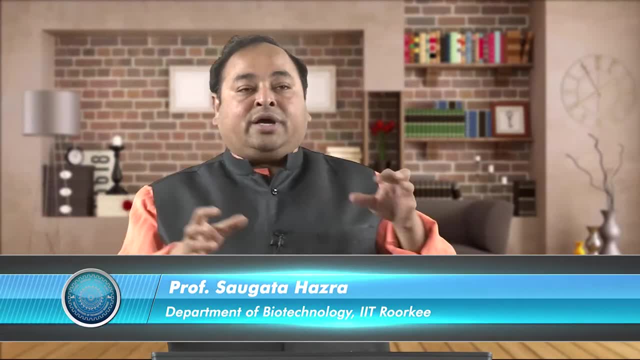 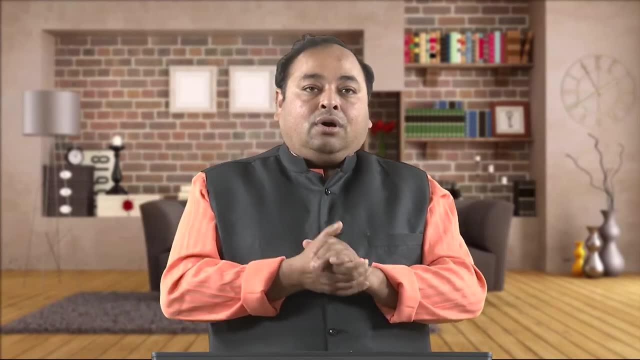 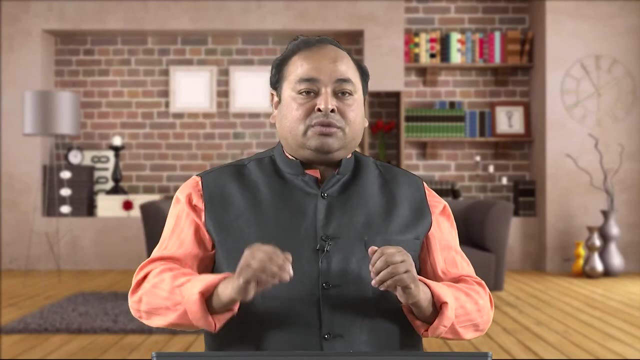 of Bravais lattice, which is having 14 crystal, to a 7 crystal system, which is there. the space groups we talked about And we end up understanding the fact that in protein there are 65 space group instead of 230 because of the chiral environment present in protein. 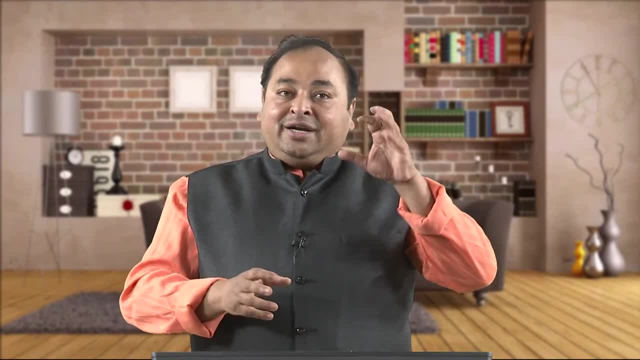 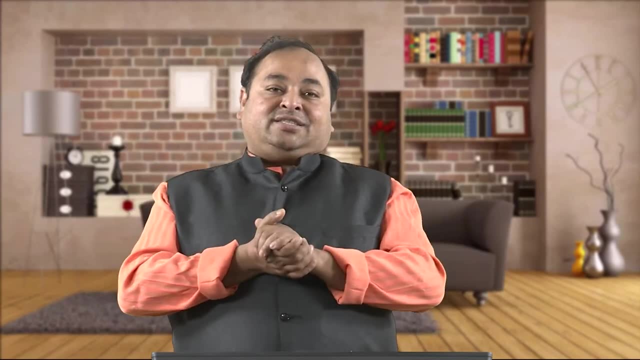 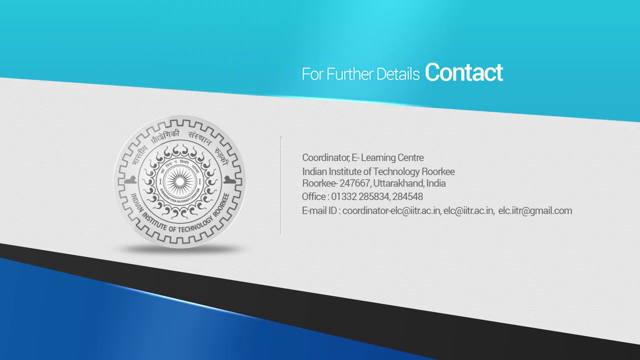 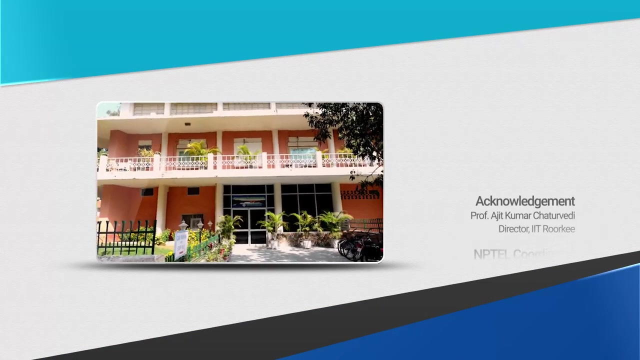 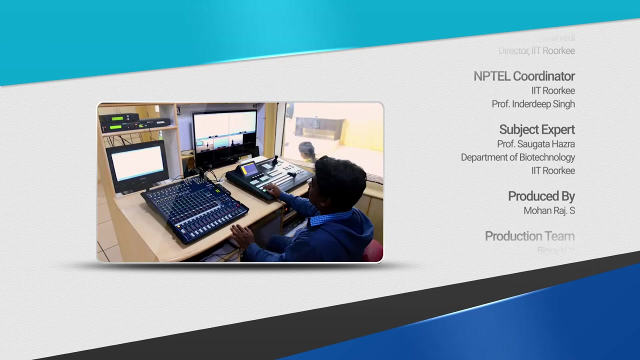 From here we will shift from direct space or real space to a reciprocal space. We will talk about Miller indices in the next class. Thank you very much. Thank you.